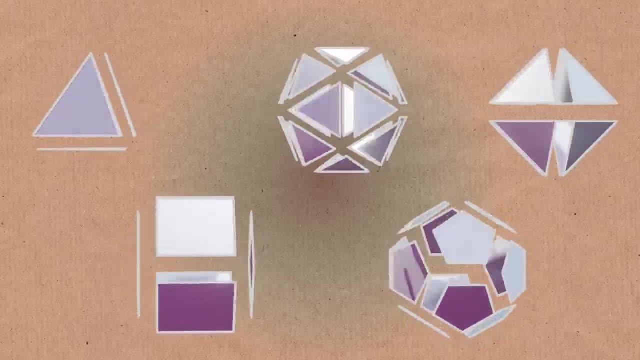 The other ones are all squares or triangles. The dodecahedron is made up of pentagons. It's made up of 12 pentagons. Three of them come together at each corner. So that's it. Those are the five. 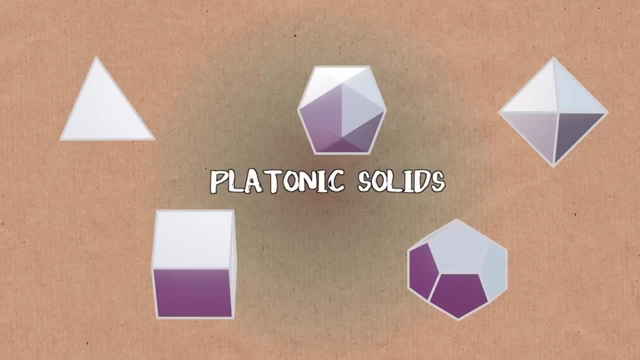 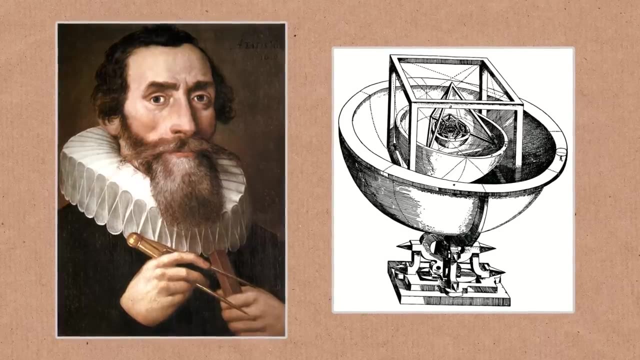 And they're known as platonic solids. They've played a big role in people's imaginations of mathematics and of art and of science. Kepler famously guessed that there might be these celestial arrangements of the platonic solids which the planets live on. Turns out that isn't the case. 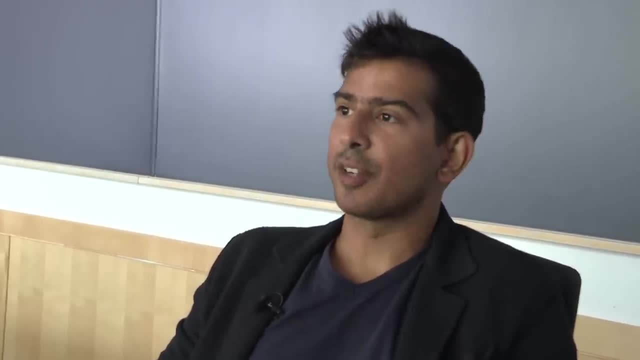 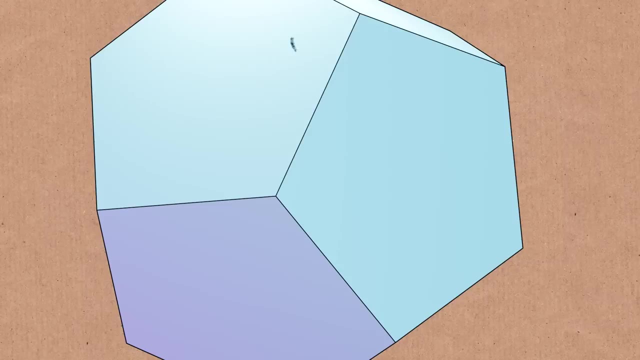 I study the geometry of surfaces, I like to think about the surface of these objects. When I say the surface of these objects, I want to think about what it would be like if you were a little insect living on one of these things. What would your experience of the world be like? Presumably insects living on the surface is the same for all the platonic solids, though, isn't it? It's like living on a sphere, except you've got pointy bits. You would think so, But the pointy bits turn out to make a difference. 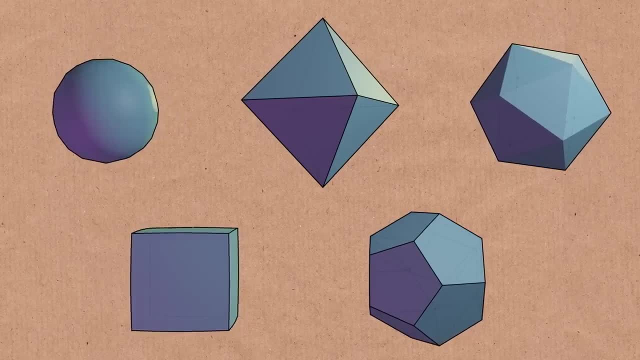 From the point of view of what's called a topologist, somebody who thinks about what we consider sort of rubber sheet geometry, all of these would be spheres If you sort of blew up and sort of tried to make this as well-rounded as possible. 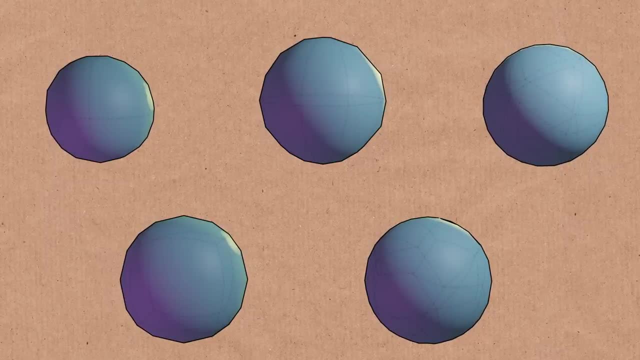 this would become a sphere. But I really do want to think about the pointy bits. Imagine, on one of these platonic solids there's a house. on each corner where a mathematician lives, At each of the vertices there's a house. 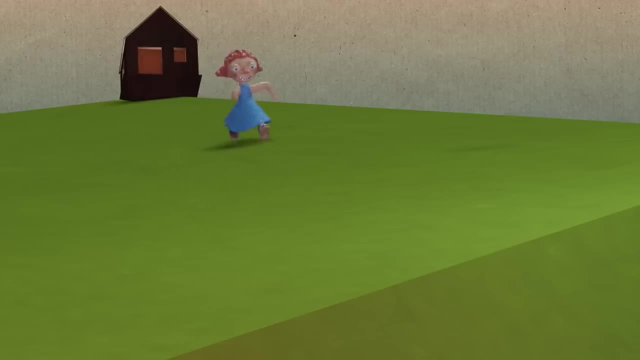 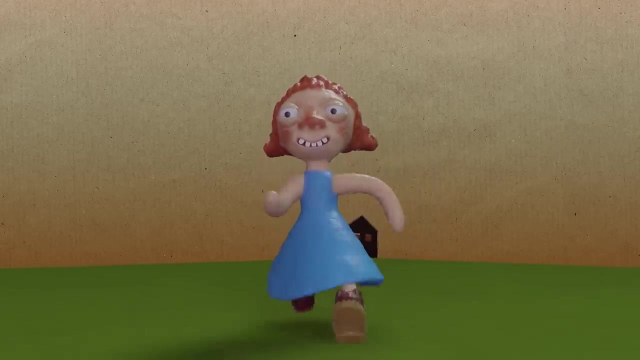 And now let's say you have your mathematician living at one of these houses and she's an avid jogger. Every morning she likes to go for a jog. On the other hand- you know it's morning- She doesn't really feel like seeing any of her neighbors at this point. 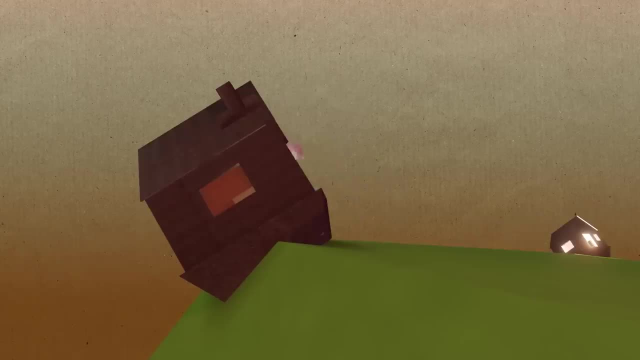 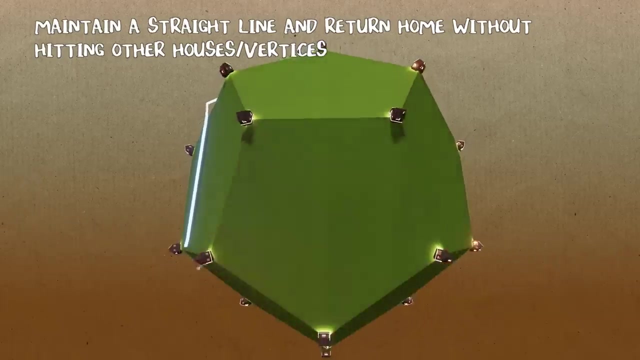 She wants to go for a jog, She wants to come back home, to where she started, And she doesn't want to run through certainly any of her neighbors' houses. She would like to go on a path and she doesn't want to have to sort of retrace steps or anything like that. 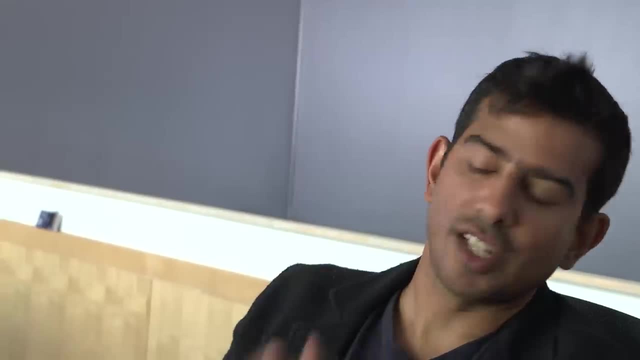 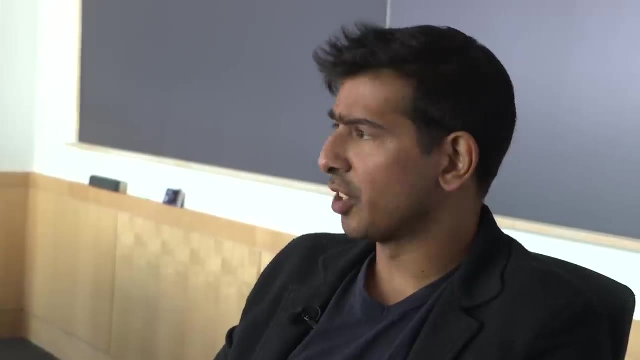 She just wants to go straight and come back to where she started. We call this maybe the antisocial jogger problem, Another framing of it if there's this classic children's book, The Little Prince, And in one of the central tensions in The Little Prince, 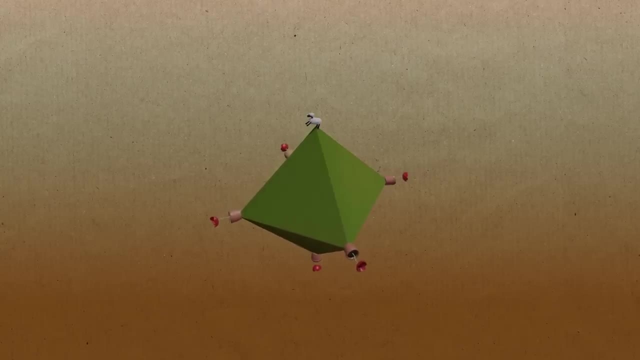 other than the loss of childhood innocence. the prince has a sheep on his planet and a rose, And he wants to prevent the sheep from eating the rose, So we could think about this generalized problem, as the prince and the sheep live at one corner. 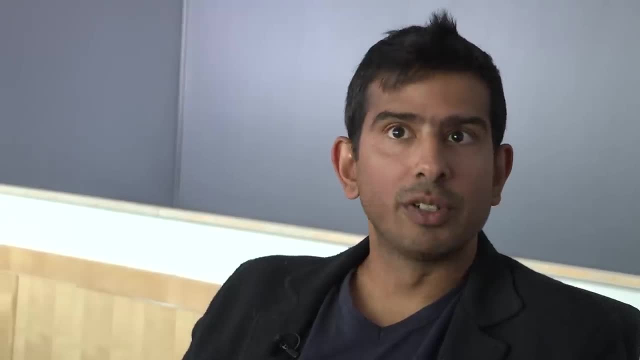 and there's a rose at every other corner. And the prince wants- he's a good pet owner, responsible, wants to take his sheep out for a walk every day, But not walk it past the rose, because then the sheep will eat the rose. 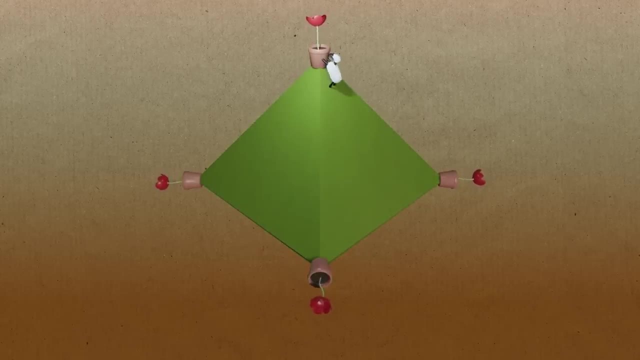 Can he do that? Can he do that on a loop? So it's kind of like you almost want to make like an equator type shape. So it's a closed loop. It's like an equator or a longitude line or a latitude line. 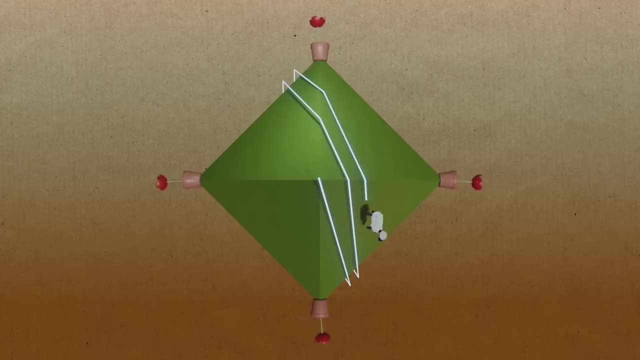 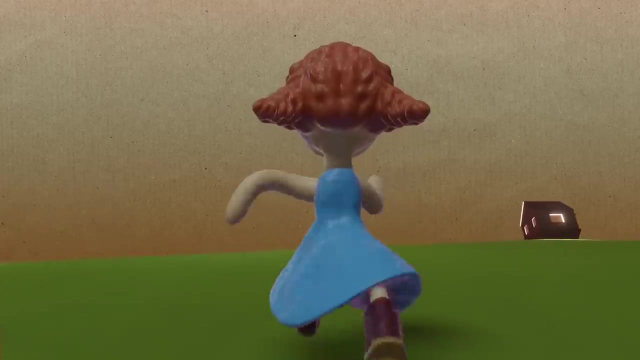 We're not asking for it to cut the thing in half. We're just asking to start at one corner, go on a straight line. You never turn, You never pass through another corner. You might say what happens when you hit an edge. 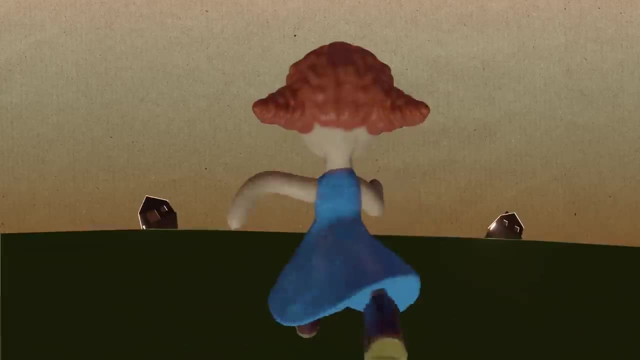 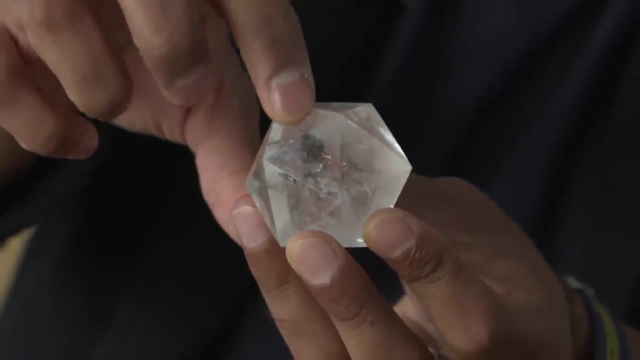 But it makes perfect sense to go straight over an edge. You can just driving your car over a ridge, walking over a ridge. It is, however, a question about what it would mean to go straight when you hit a corner. For instance, here in the icosahedron, we have five triangles coming together at a corner. 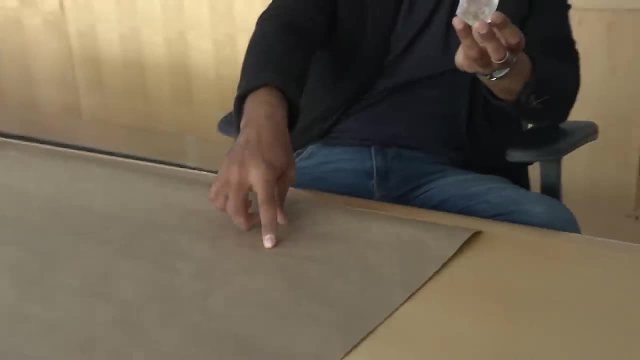 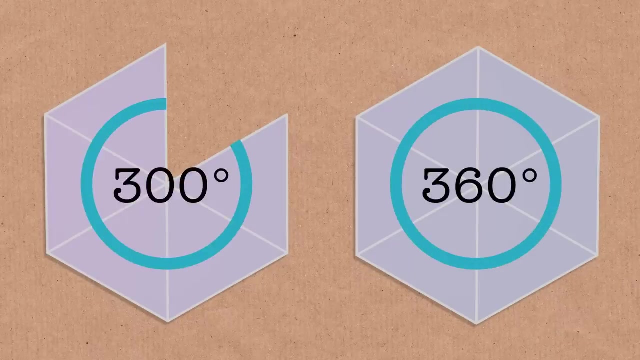 If you think about a flat piece of paper, you'd have to have six, You'd have to have 360 degrees. Here I have five triangles, so I only have 300 degrees worth of angle. So this is another reason we don't want to pass through corners. 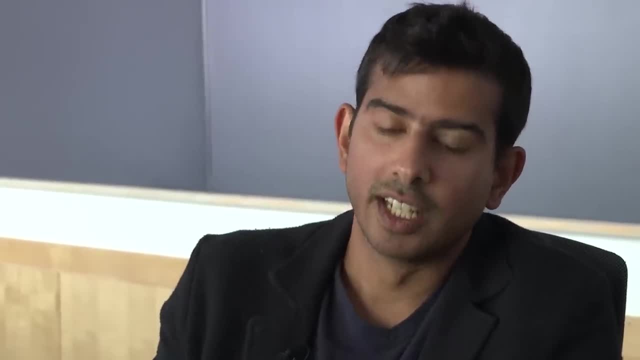 because it doesn't make really sense to talk about what it means to go straight through a corner. It makes sense to go straight over a side, but it doesn't make sense to go straight over a corner. So the paths we want start at a corner. 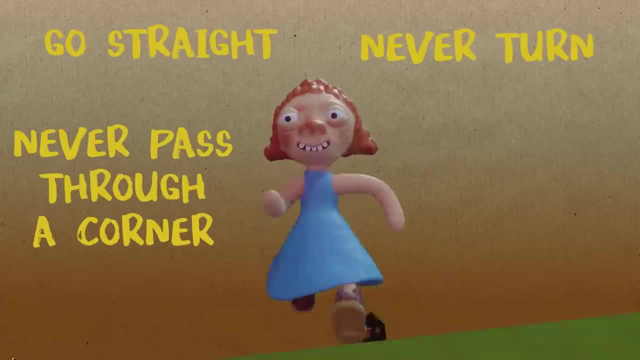 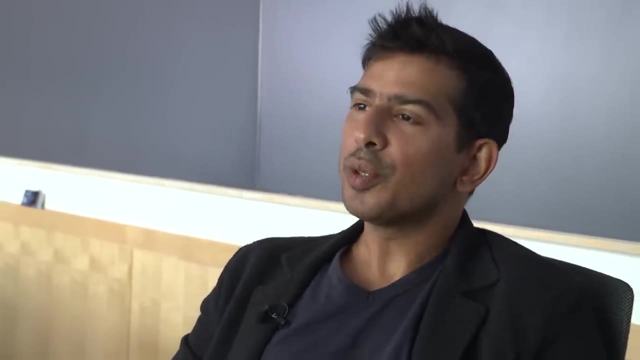 go straight, never, ever turn, never pass through a corner and come back to where you started. My sort of intuition is: there must be thousands and millions of routes you can take, or are there none? So you're right, you're right and you're right. 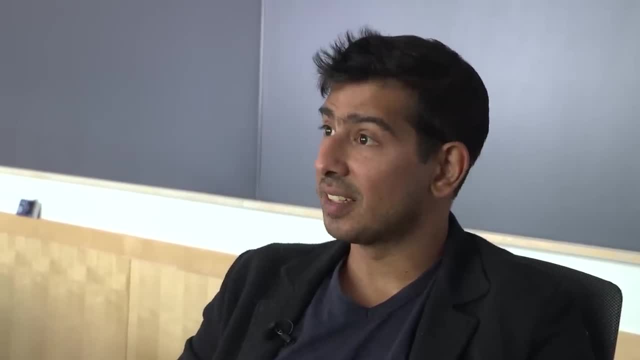 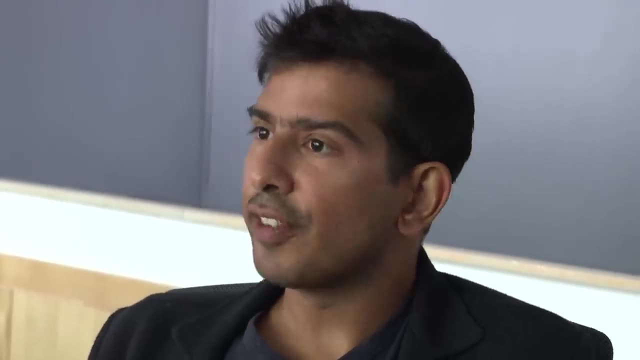 So for some of the platonic solids, it's extremely easy to see that you can't do it, So I'm going to first show you for the tetrahedron- This is something that's been known for a long time, In fact- the tetrahedron, the octahedron, the cube and the icosahedron. spoiler alert. 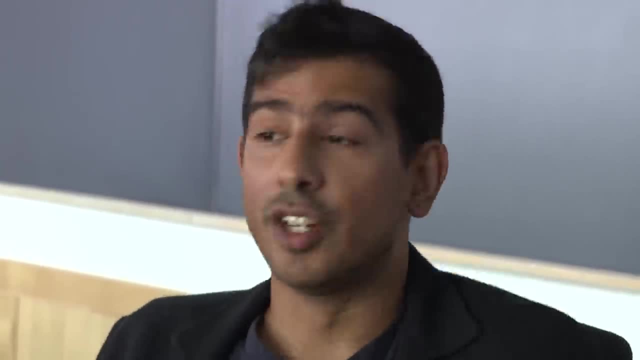 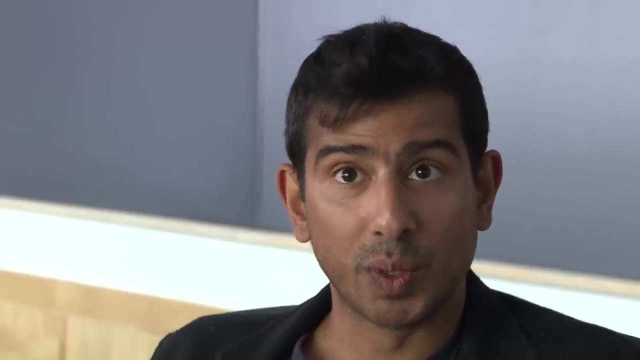 you can't do it on any of them, But people didn't know whether you could do it on the dodecahedron, And that's the question we ended up answering. We showed not only could you do it, there's lots and lots and lots of ways you can do it. 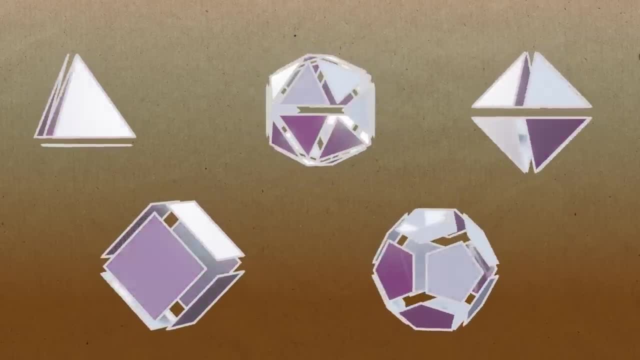 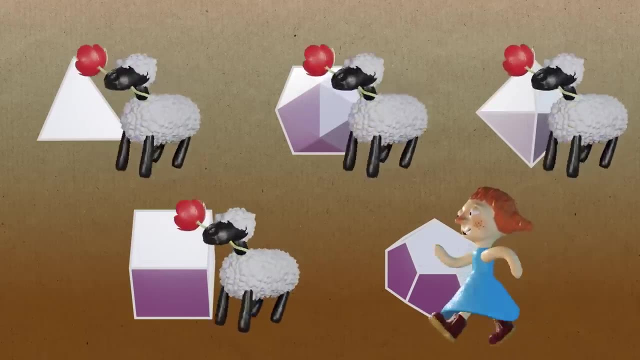 The dodecahedron is the only one you can take your sheep for a walk on without having your roses eat. It's the only one you can be an antisocial jogger on without having to retrace your steps With all of the other ones: the tetrahedron, octahedron, cube and icosahedron. 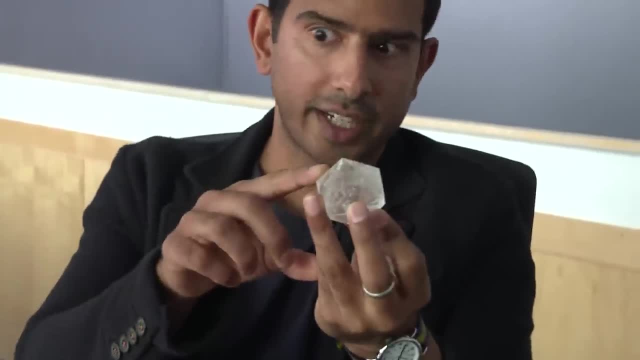 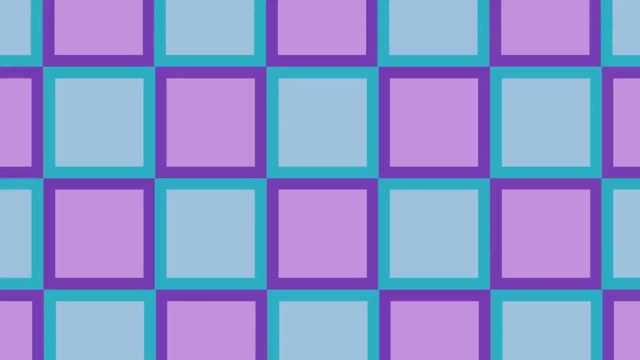 the shapes that make them up. in the icosahedron case trine, in the cube case squares, in the octahedron and tetrahedron triangles. they end up tiling the plane. You could tile your infinite bathroom floor with copies of these things. 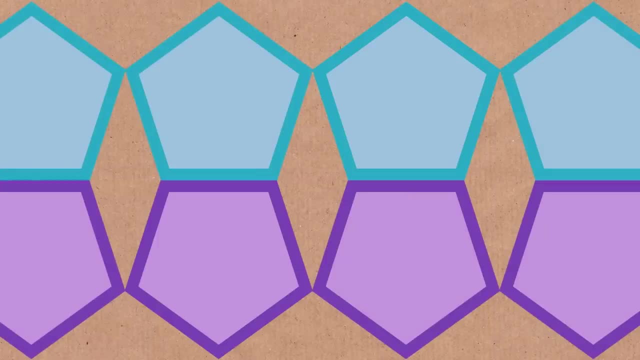 You can't do that with a regular pentagon, Four of them. it was impossible and that's long been known. That's long been known. We didn't know for the dodecahedron. We didn't know for the dodecahedron. 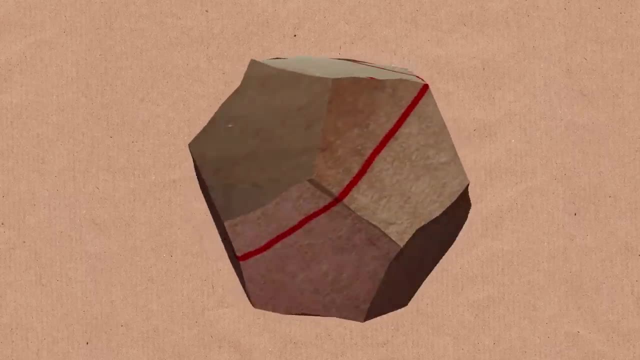 How is that possible? Couldn't I just make a dodecahedron out of cardboard, get a sharpie and draw a line and think, yeah, there you go. It was easy. So that's a really good point. You probably could do that. 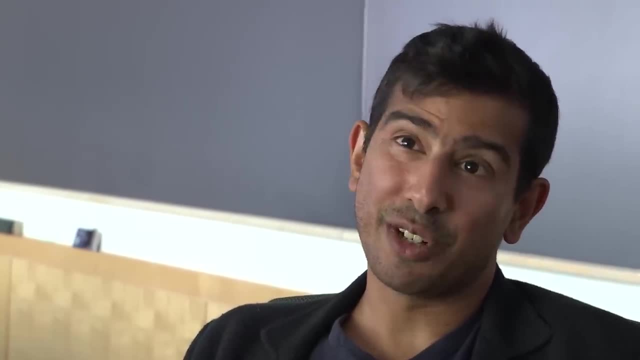 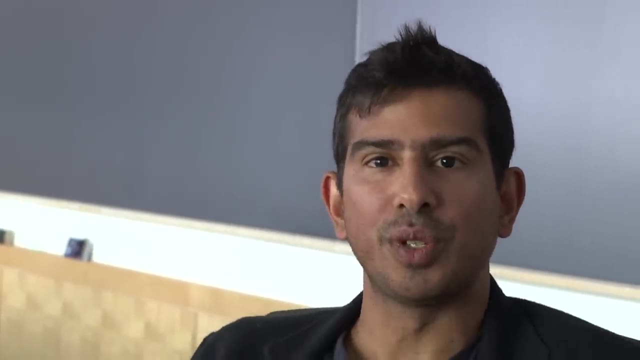 How is that possible, However, you wouldn't be sure that what you got was an exact mathematical trajectory. Maybe the thickness of your sharpie, maybe there is one that's a little bit off Even on the other ones. probably by nudging a little bit you could do that. 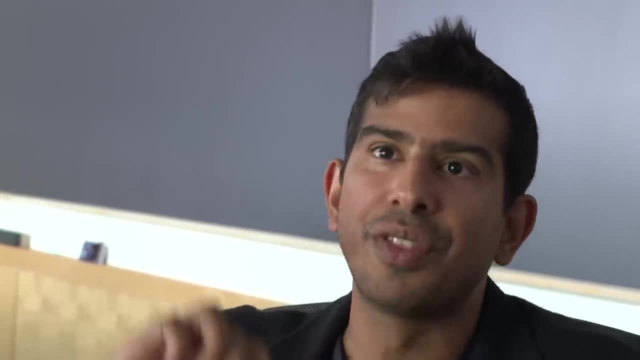 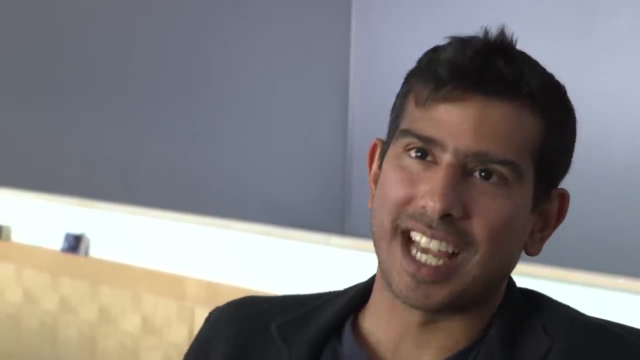 So we wanted an exact straight line with no width, no thickness, coming back to where it started: That little thickness of your marker. you wouldn't know whether that actually gave you that exact mathematical answer or not. So I take it from that that the paths that do do it. 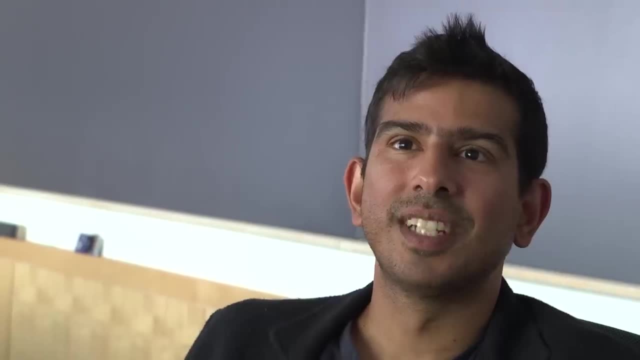 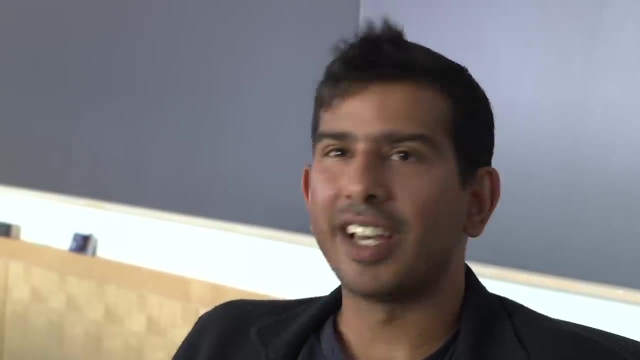 that we're about to talk about only just miss the vertices. then, Yeah, Yeah They. surprisingly enough, the most simple one we found is one that you would look at and you would kind of draw by eye To prove that it is. one though is a little bit trickier. 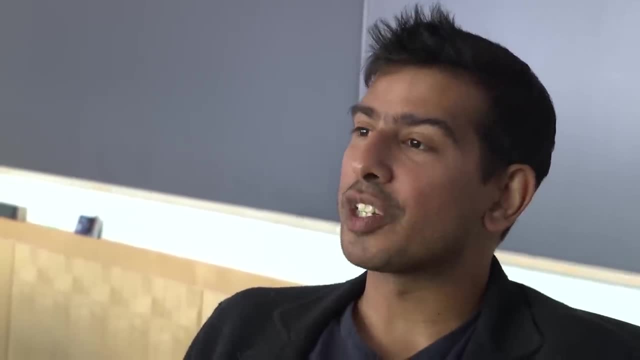 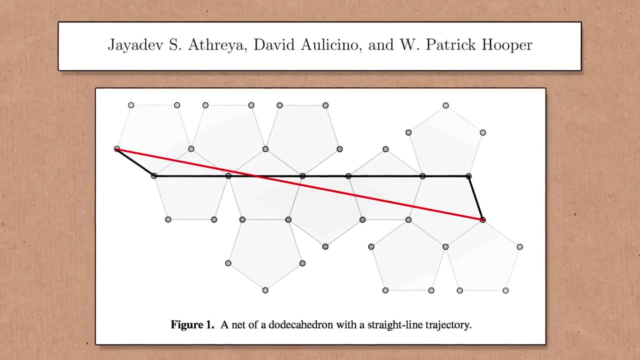 It's shockingly simple to us. This is what made this project so much fun. This was with my friends, Pat and David. We found a beautiful, simple, elegant solution, And it also has the advantage that it's visually very pretty. I want to prove to you that, at least in one of the cases that you can't do it, 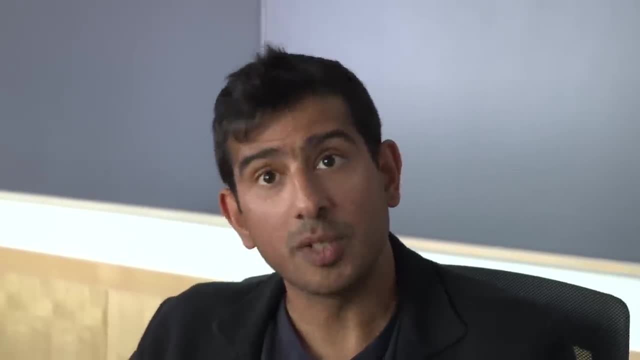 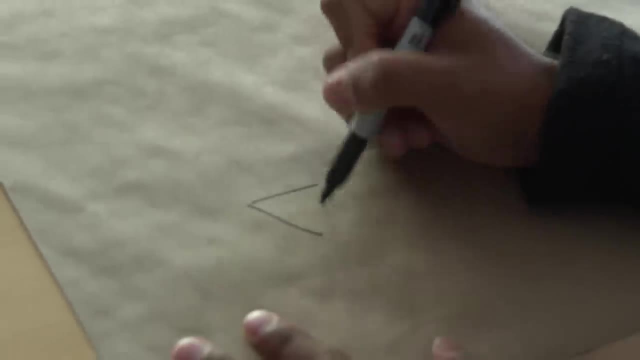 I want to show you, for the tetrahedron, that you cannot do this, because it illustrates an idea that we're going to use for the dodecahedron. It illustrates the idea of what's called unfolding. Let me start by drawing how I think of a tetrahedron. 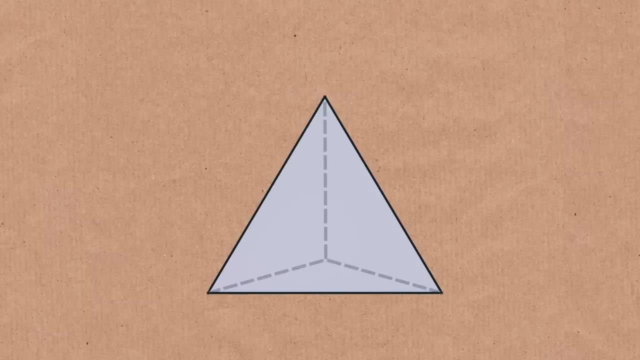 So a tetrahedron, of course, is this kind of pyramid shape with a triangular base, But, like I said, I like to think about the experience of kind of living on the surface. I'm going to draw you a diagram to make a tetrahedron out of a flat piece of paper. 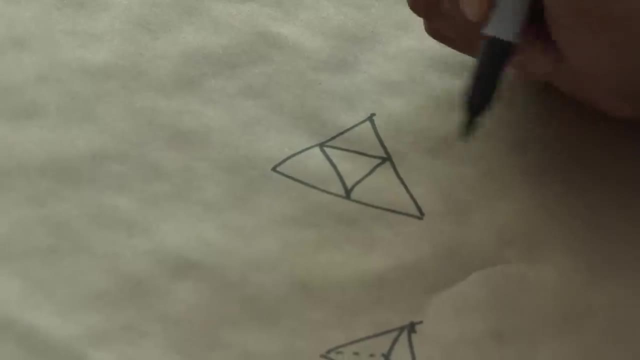 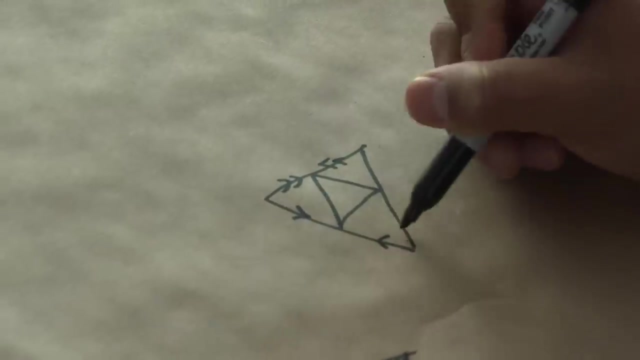 This is called a net. I'm going to draw a big triangle, sort of cut up into four, And then I'm going to draw you gluing instructions. So gluing instructions is that side gets glued to that side, That side gets glued to that side. 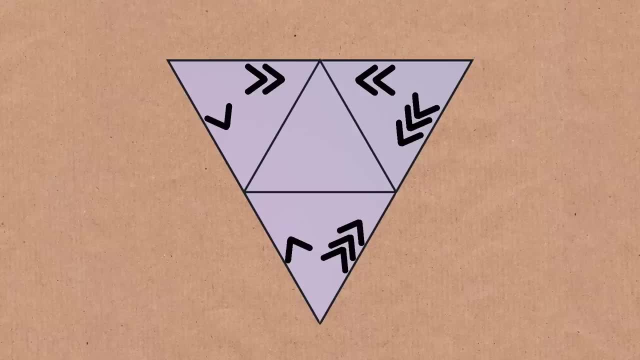 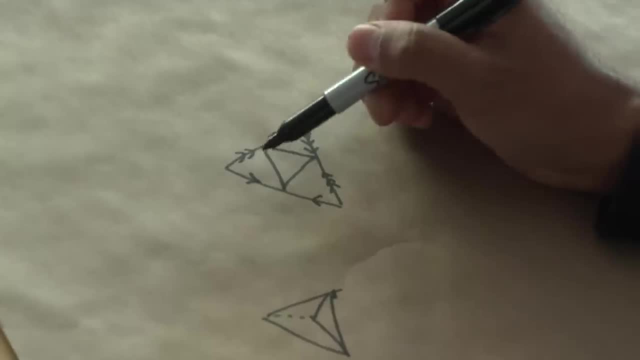 And then that side gets glued to that side. If you were to fold up, you fold it along these internal edges. these guys end up glued up And notice, the direction of the arrows is important here. You know, going this way gets glued to going this way. 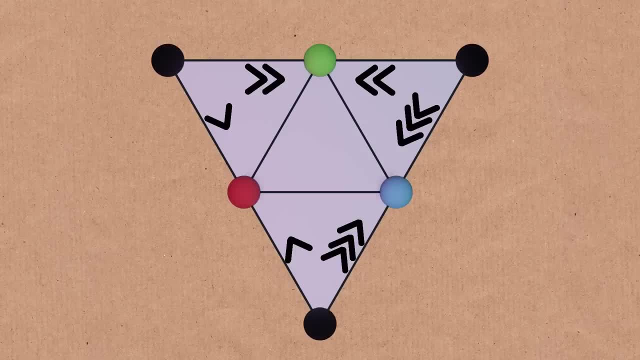 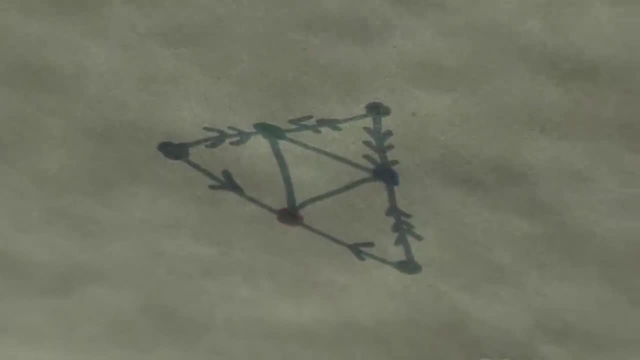 And now I'm actually going to label the corners. If I think about folding this guy up the very top, all these three guys end up folding up to this one point. So these are the four corners, And what I want to do is I want to draw a path that starts at one of these colored corners. 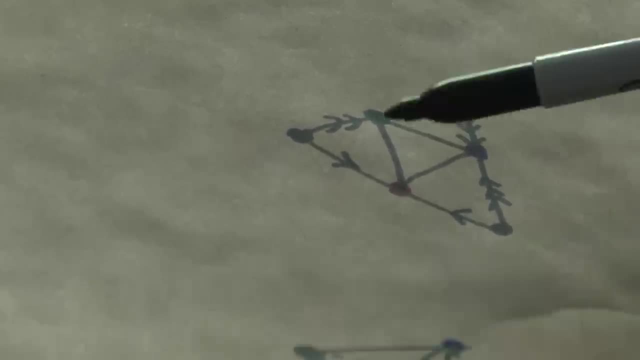 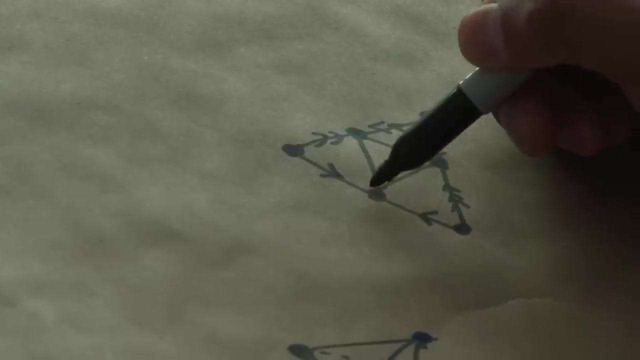 comes back to itself Without passing through any of the other corners. I could try and draw it on here, but it might be easier to draw on here and kind of a map of this thing where I just follow the identification. So you know, for instance, if I were to start here and kind of go like that: well, now I'm. 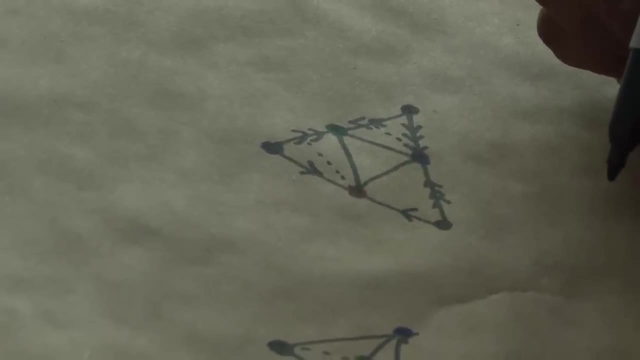 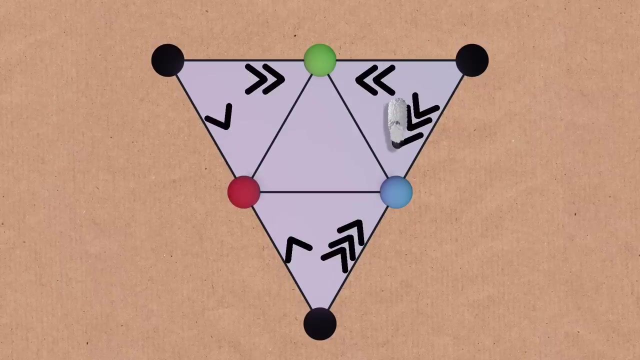 here and I would come like that: Uh oh, I've run into the blue right. That's something I don't want to allow. To make this even clearer, notice here: I was going along this way and then I had turned around 180 degrees. 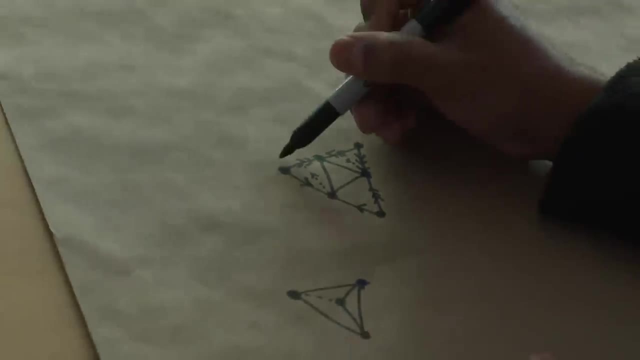 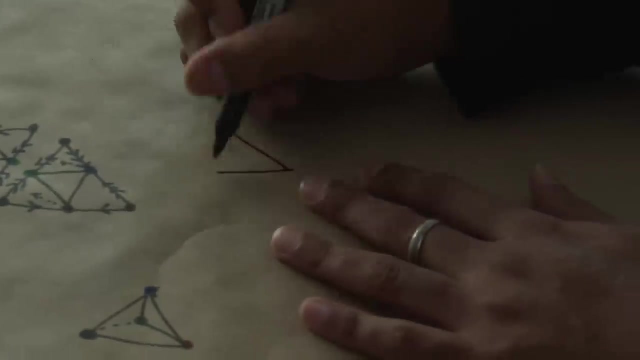 Let me make a drawing where I never actually have to turn around. So I'm just going to draw a copy of this guy rotated by 180 degrees, And now I get a rhombus. I'm going to draw that rhombus for you without any of the distracting internal lines. 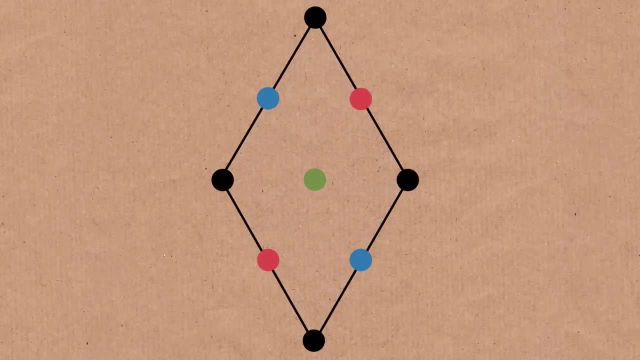 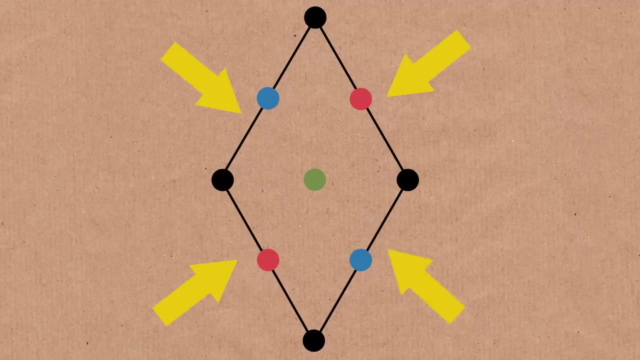 But I am going to keep drawing these internal corners. It's very pretty decorated rhombus, But it's not just a rhombus. Notice the left side here is the same as the right side and the top is the same as the bottom. 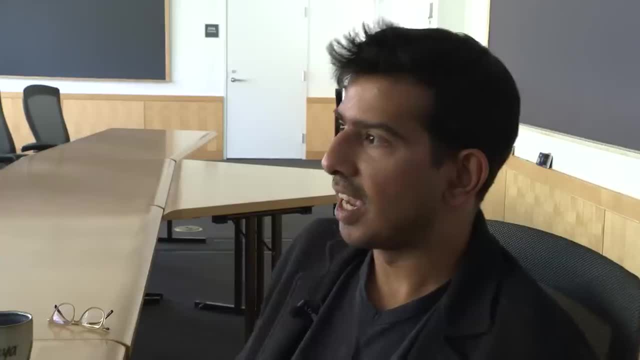 You know, if you ever play the computer game Pac-Man- and of course, as I get older and older, less and less people understand that reference. But most many computer games and you play on a screen, you go off one side, you come. 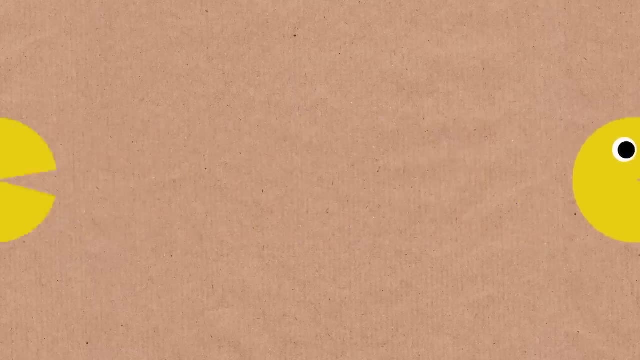 up the other. It's kind of this repeating world. You go off the top, you come up the bottom- Asteroids, Asteroids. In fact that's a better one, because Pac-Man can only move parallel to the sides And asteroids. you can kind of move in any direction. 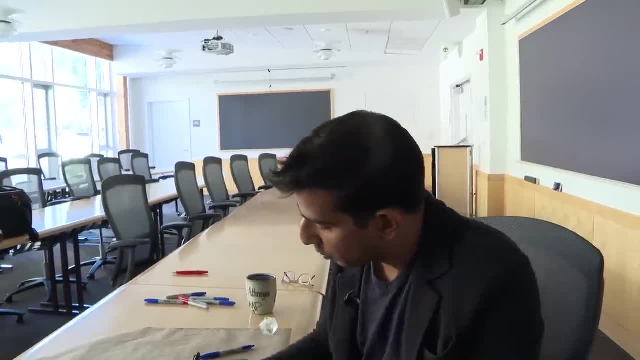 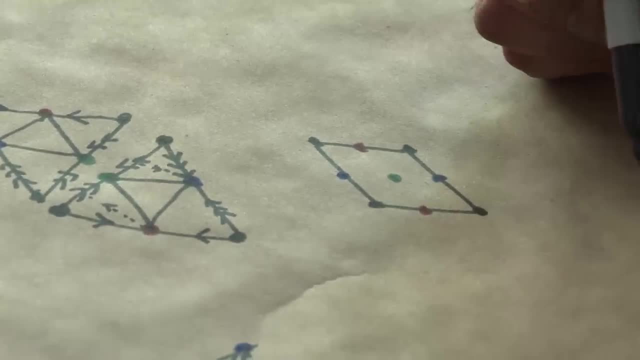 So imagine playing asteroids on this parallelogram board. What we want is we want an asteroid trajectory that starts at one of these colored corners, goes straight, goes through these things, never passes through another corner and comes back to where it started. But I'm actually now going to do one more piece of unfolding. 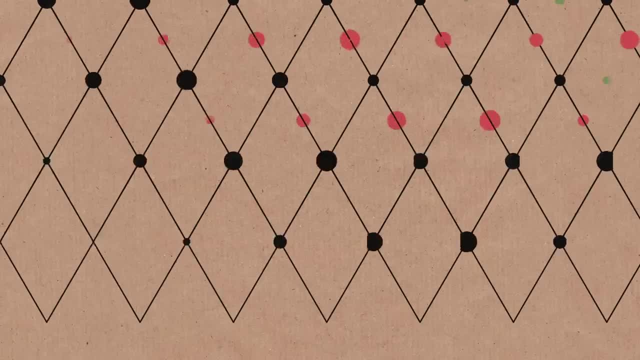 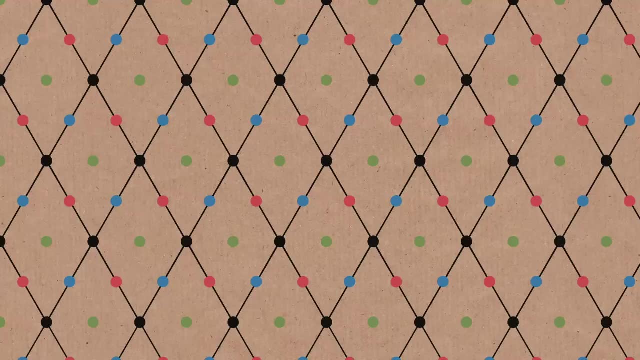 I'm going to draw. this picture is kind of repeating forever. I can tile an infinite room with copies of this rhombus. And now what you want to do is you want to draw a straight line Starting at one color, ending at the same color, without passing through any of these. 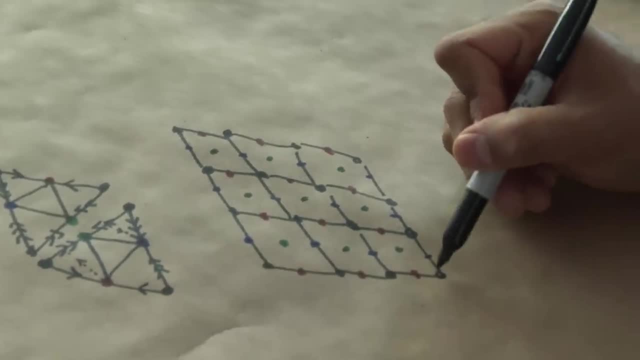 things. But notice, let's say I wanted to go from black to black. If I want to go from black to black, well, I could try and go diagonally, but the green blocked me. I could try and go horizontally, but this blue blocks me. 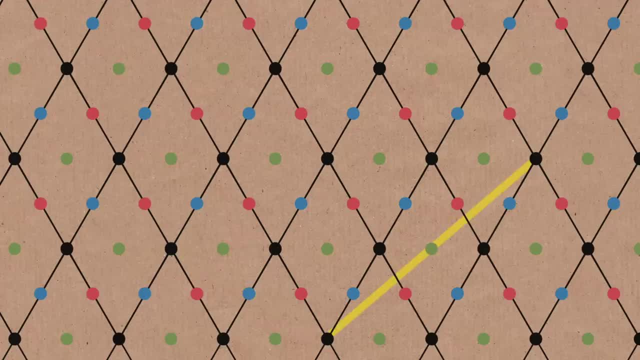 I could try and go vertically, and the red blocks me. No matter what I do, I'm blocked, And so these points block each other from accessing themselves. For the other platonic solids other than the dodecahedron, the unfolding isn't quite. 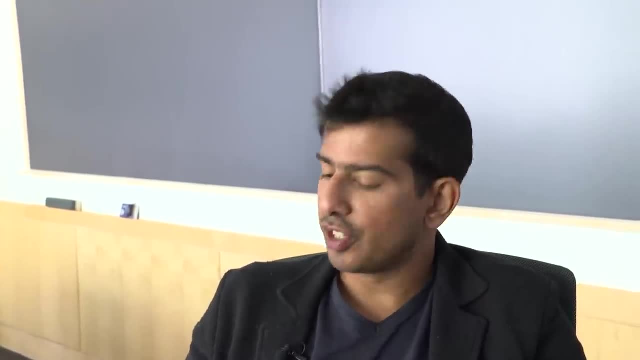 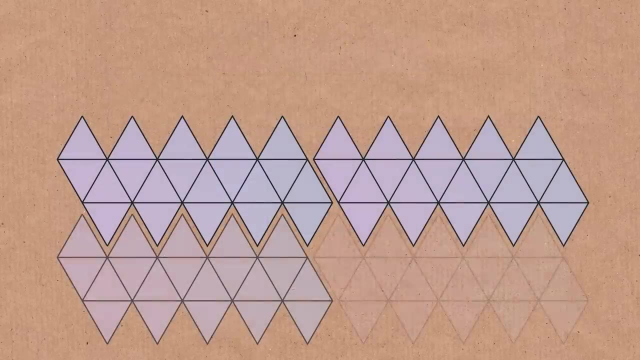 as simple. You need to do more copies. So, for instance, for the cube, the net for a cube is something that looks like a cross that you put together and you need four copies of that. For the icosahedron, you need six copies. 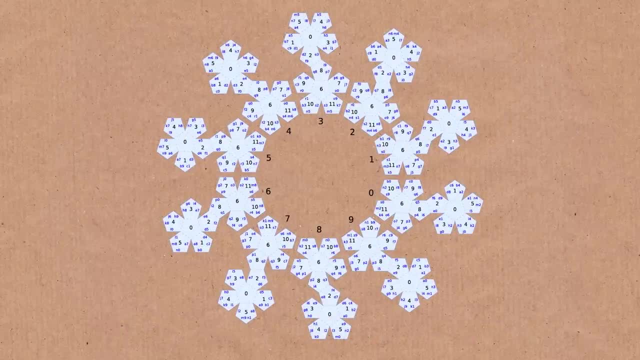 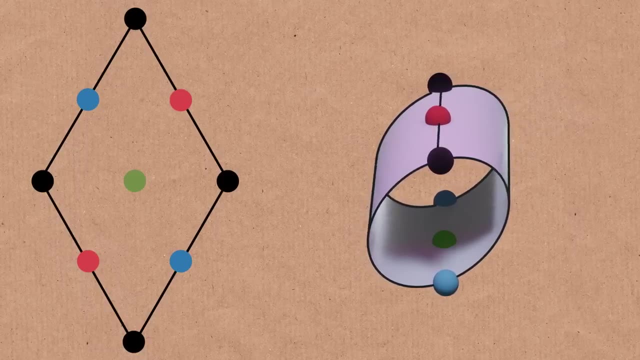 For the octahedron you need three copies, For the dodecahedron you need 10.. There's also something really beautiful going on here If you think about taking this parallelogram and gluing opposite sides. if you glue the. 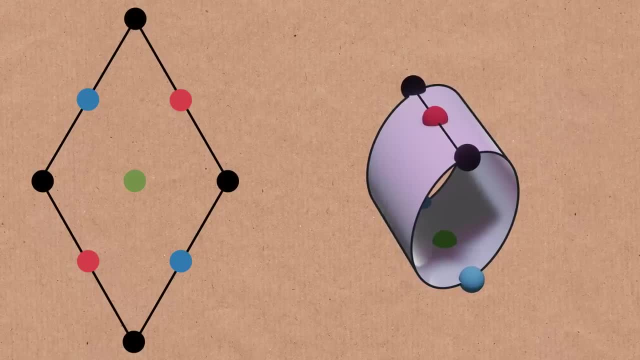 left to the right. you get kind of a sheared tube And then you glue the top and bottom of the tube. you get something that looks like a donut. This is called a torus or a genus. This is called a genus. 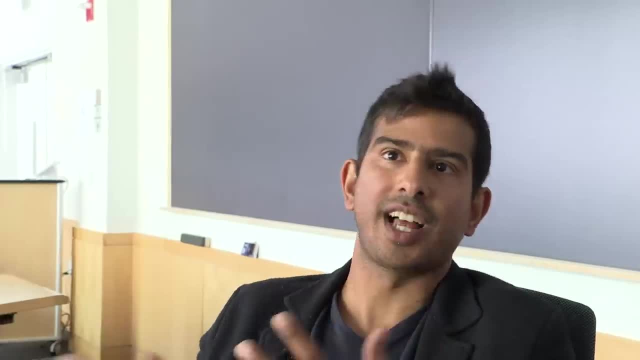 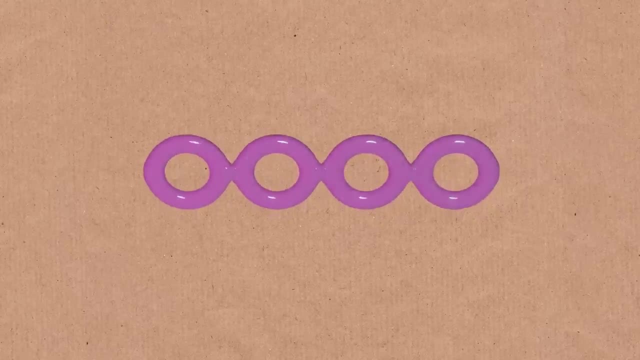 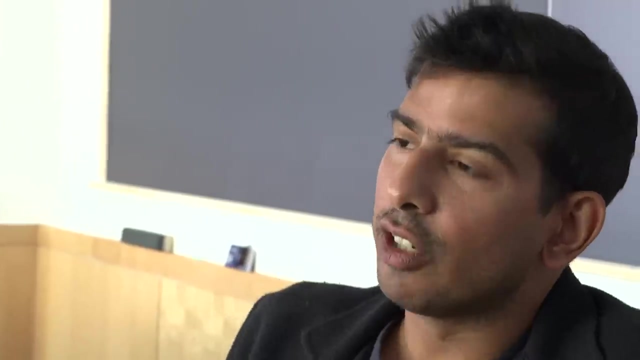 They're not so complicated. the other ones: The octahedron gives you a genus 4 surface, the cube a genus 9 when you do this unfolding procedure. This unfolding procedure leads to things that aren't too terribly complicated, until you get to the dodecahedron, where the resulting surface. if you were to play Pac-Man on this, 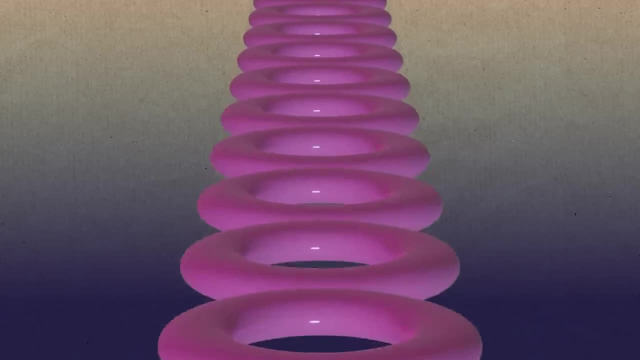 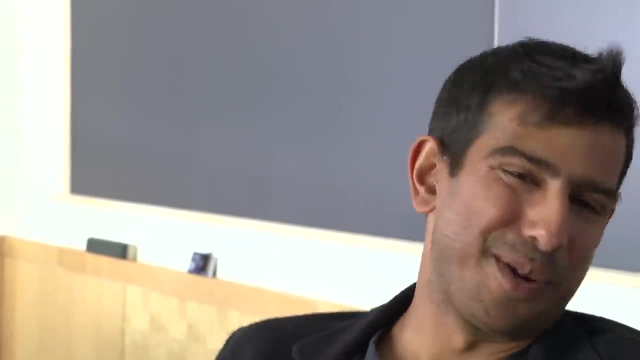 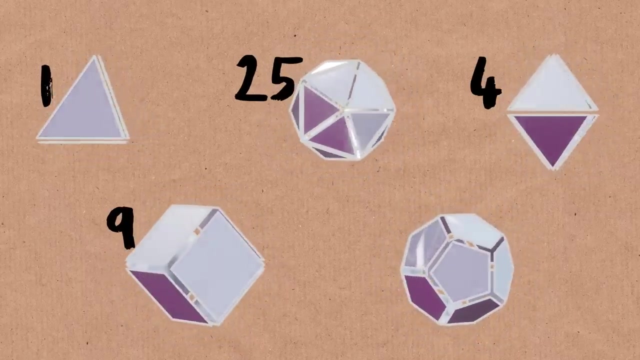 crazy surface. it would be like living on a surface with 81 holes, And no, it's not an accident that the number of holes is always a square. We can talk about that at some other point. It goes 1 for the tetrahedron, 4 for the octahedron, 9 for the cube, 25 for the icosahedron and. 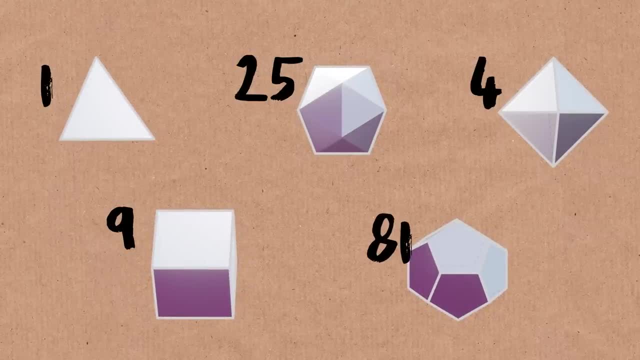 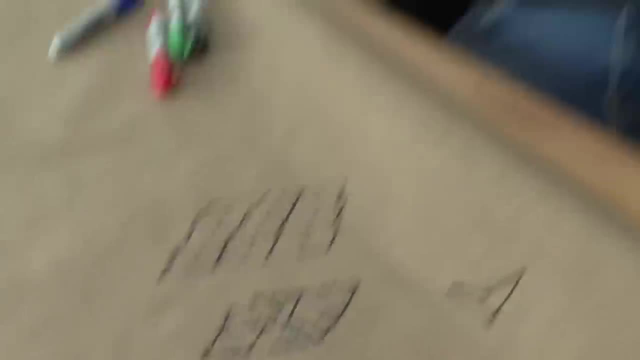 then 81 for the dodecahedron. The dodecahedron, it was completely open. But the idea, the key idea from this is that the right place to look was in the unfolding, Because in the unfolding what we traded is we've gone to a much more complicated shape. 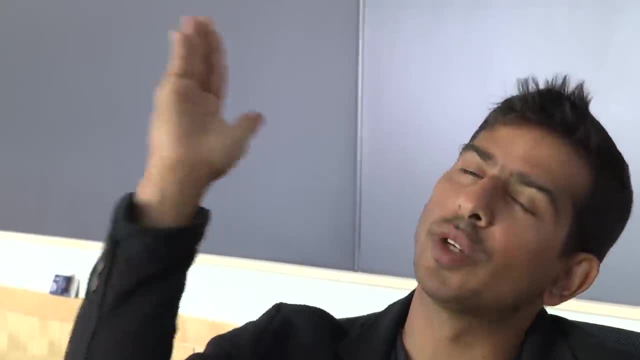 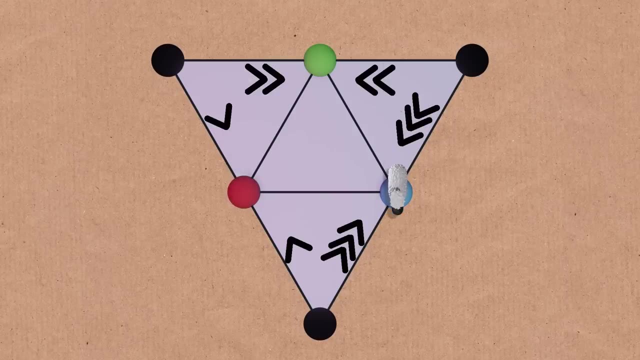 but now the trajectories we care about are just straight lines And then once we go through a side we just keep going straight in that direction. We never have to change direction. Here we'd have to turn 180.. On the dodecahedron we'd have to turn sort of a multiple of 72 degrees. 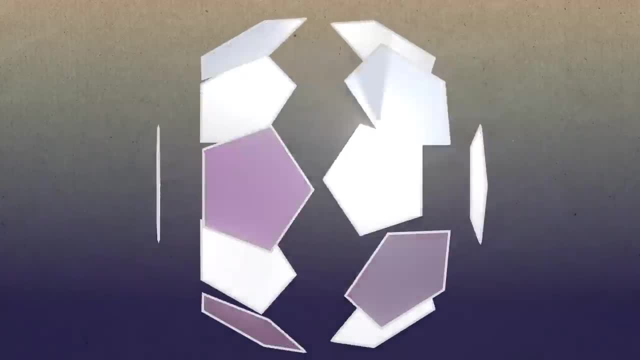 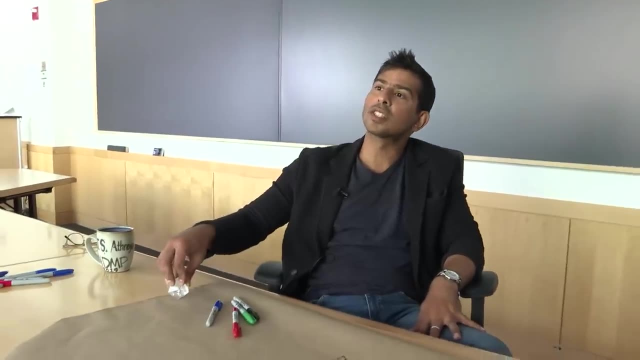 But now we're just going straight by keeping track of all the copies. What's the dodecahedron got there? What's its special magic? So for the tetrahedron you got what was called a torus. For all of these guys you get something that looks kind of like a torus. 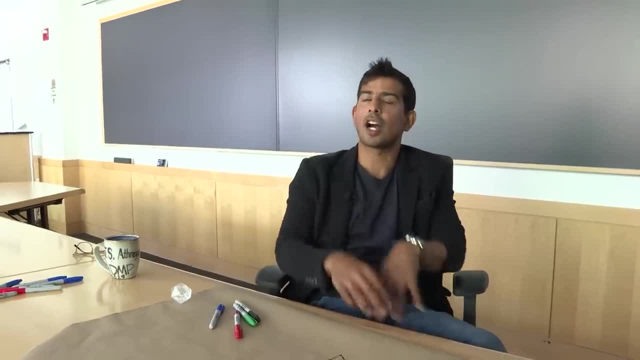 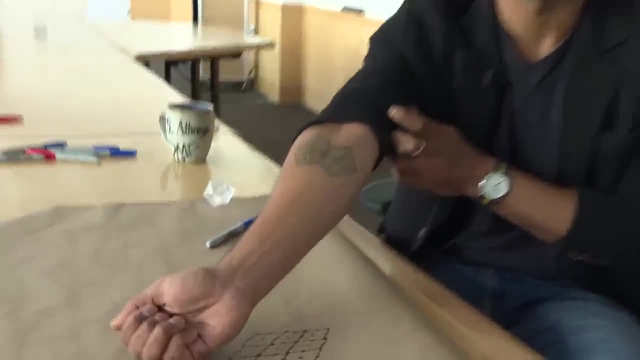 It's called either square-tiled or rhombus-tiled. It's covered by tiles- Right Tiles- of this form. The dodecahedron covers something called the double pentagon. You got a tattoo. I got a tattoo. 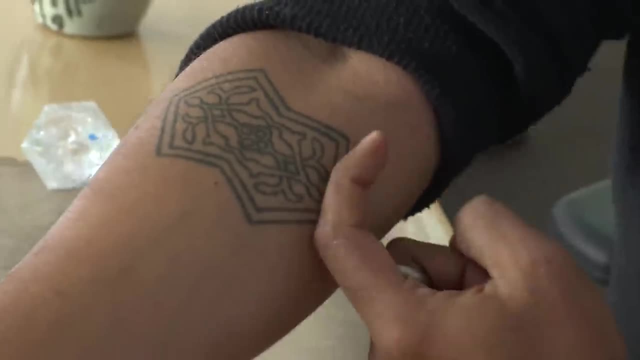 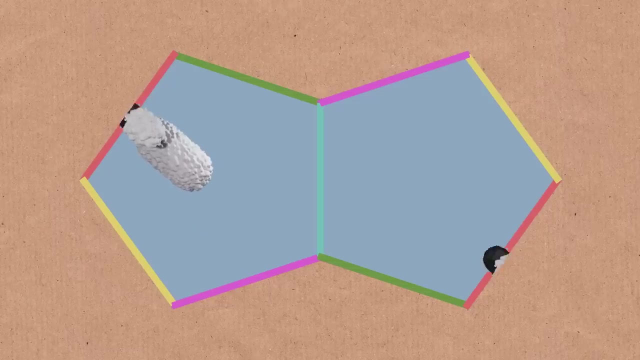 This is actually even before I worked on the dodecahedron. I had worked on this surface. So imagine playing Pac-Man on this surface. You glue this side to this side, this to this, You glue the parallel sides, So you go off this side, you come up here. 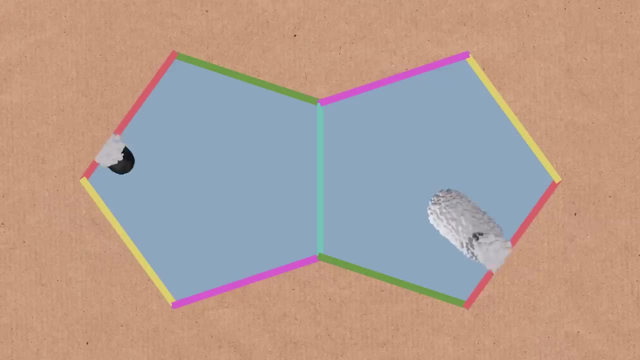 And I had studied playing Pac-Man on this before and I didn't know that it was going to be relevant to the dodecahedron. It turns out if you start with the dodecahedron, we said it started with 12 pentagons. 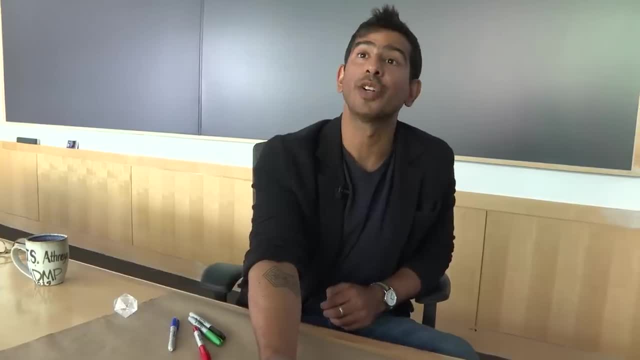 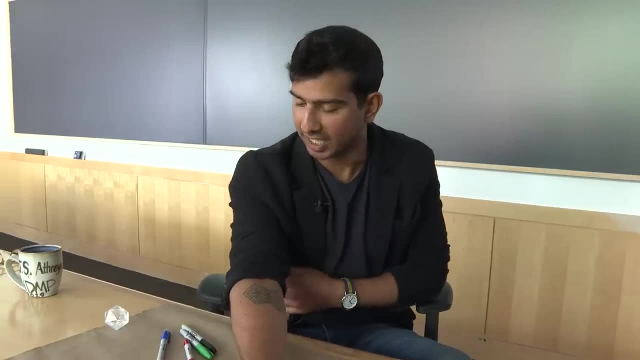 And then I said I need to take 10 copies of this. That gave me 120 pentagons In math. we call this. the construction we have is: it's a branched cover, There's 10, it's a degree 10 cover. 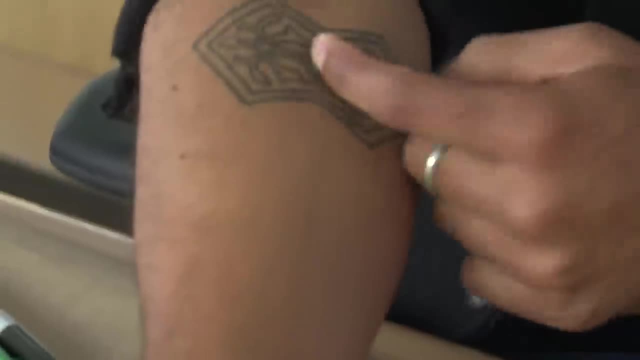 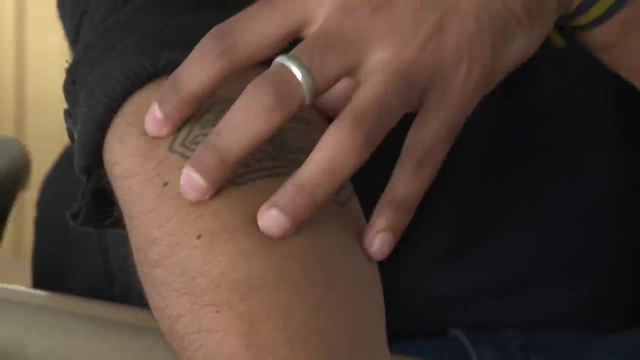 But 120 pentagons. notice, this thing is two pentagons Right. This is called the double pentagon. It turns out the dodecahedron. unfolding the thing with 120, is made up of 60 copies of this fellow. 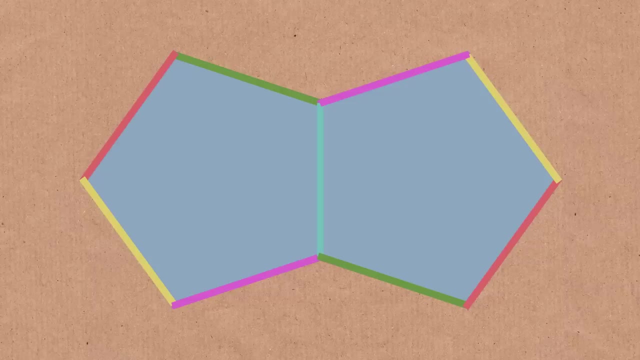 So on this fellow, if you glue these opposite sides, all the eight corners collapse to one point. So this guy gets glued To this guy gets glued to this guy, So all these eight corners collapse to one point. If we could find things on here that connect this corner to itself. 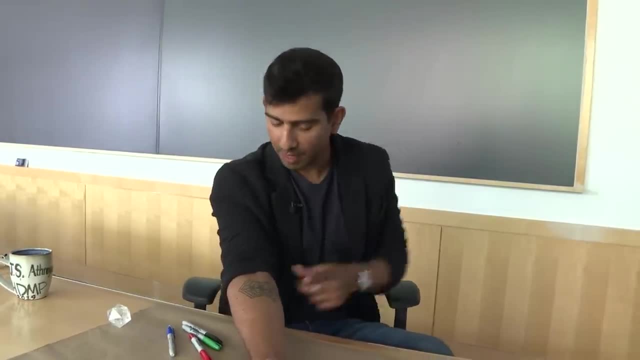 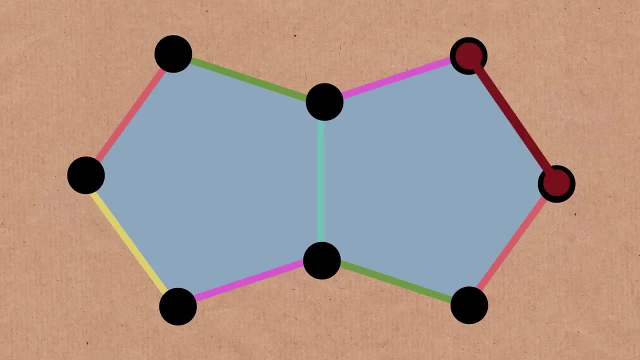 those would give us kind of candidates upstairs. Now it turns out there's kind of two different kinds of things here. There's these sides. They clearly connect a corner to itself. There's also the kind of the diagonals This guy would go across and connect to itself. 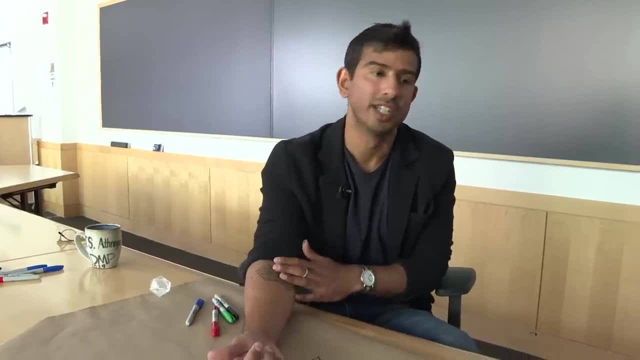 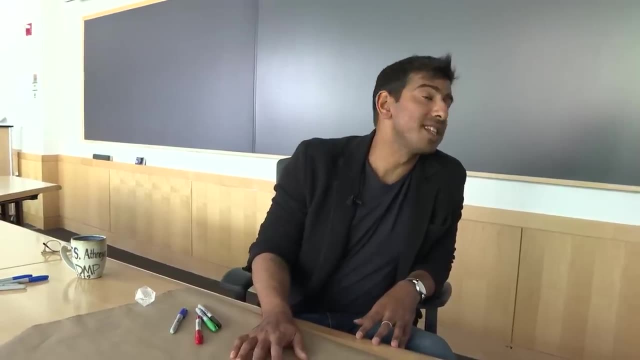 We call these the short and the long. The sides are short, the ones are long. It turns out if you kind of take copies of the short one up on this genus 81 surface, the short ones never work. They will never give you something that starts at a corner. 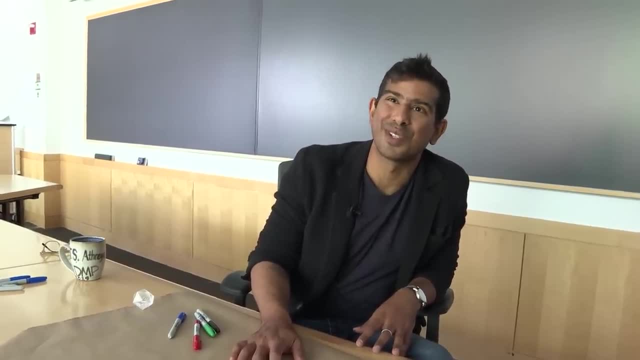 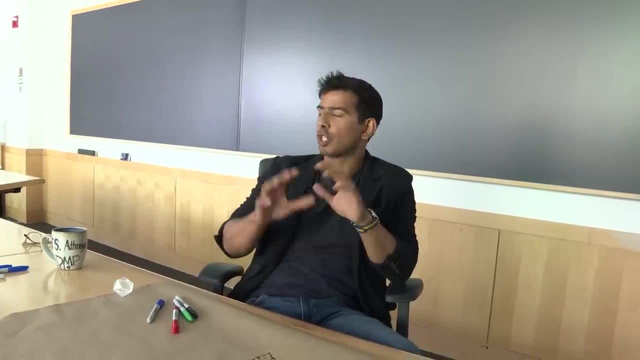 and comes back to itself without passing through another. However the long ones do. Sometimes Not all of them, And in fact up to a natural notion of equivalence which I don't want to get into too much here. you can classify the kinds of closed trajectories into 31 types. 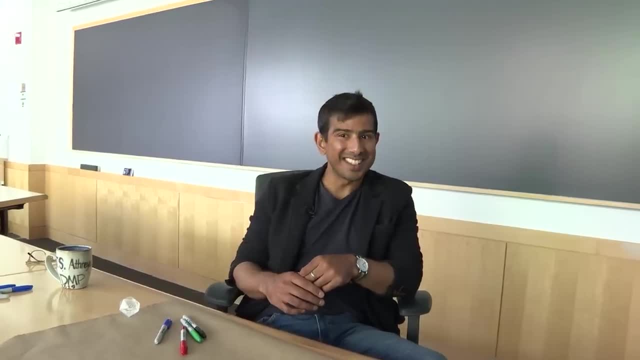 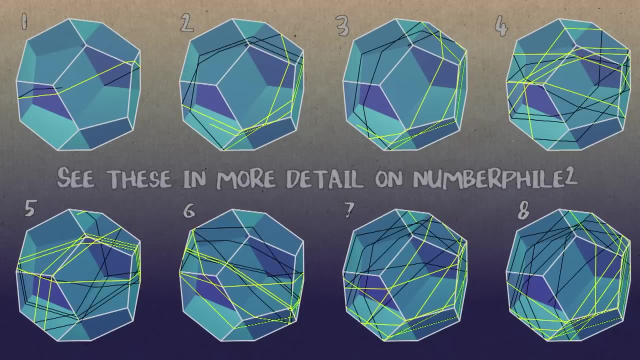 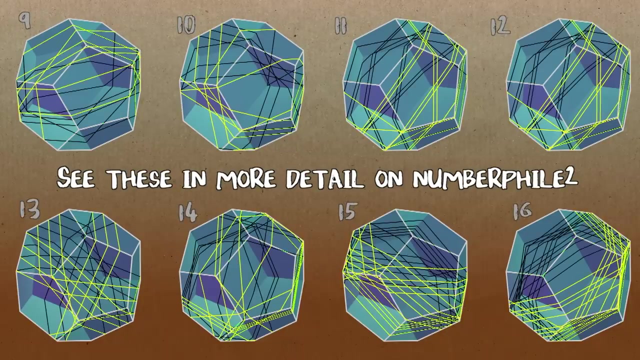 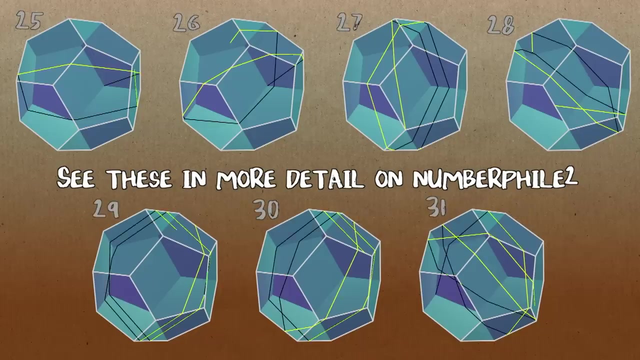 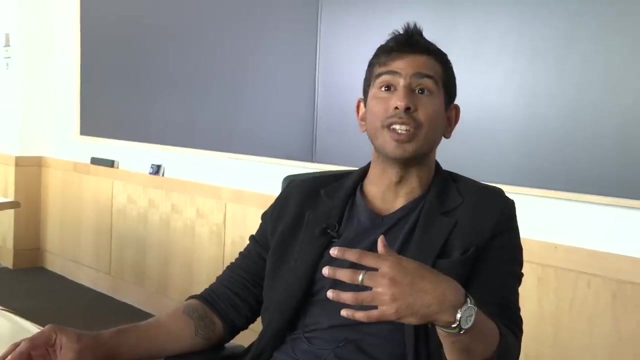 And we found the shortest guy in all of these 31 classes And we have pictures of them And we have animations of them. Of course, in each of these 31 classes actually, there's infinitely many of these, And we can in fact count them by how many there are of length less than or equal to. 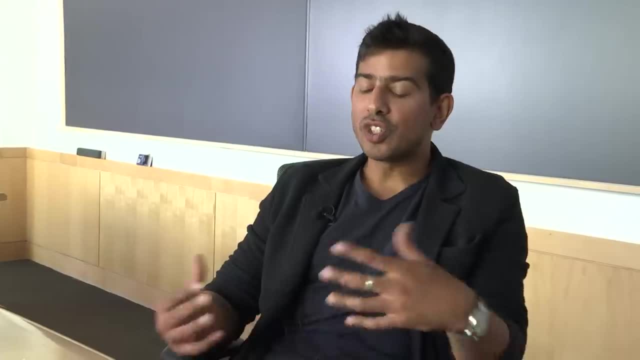 let's say 1,000.. We know how to do that as well. So we started with a question that nobody knew the answer. to Start at a corner of a dodecahedron. Can you come back to where you started? 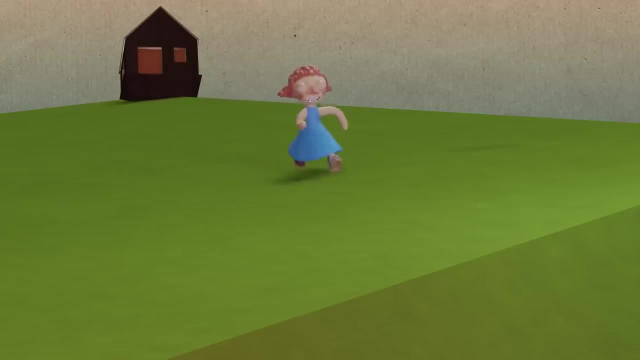 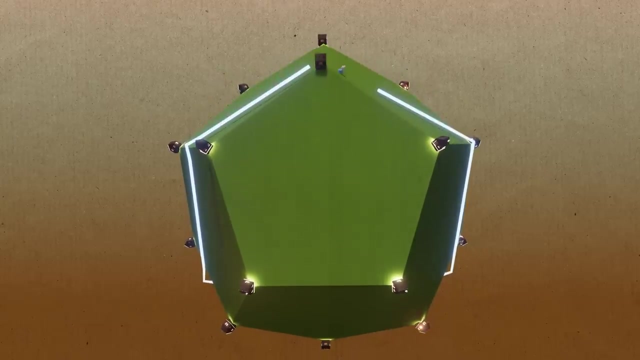 Nobody had known the answer to that. People had been thinking about that particular problem for at least 100 years. There's German mathematicians in 1906 who wrote a paper about it And we came to a very satisfying answer. The simplest answer is really simple. We have a paper, in fact, that says that the answer to this question is very simple. We have a paper, in fact, that says that the answer to this question is very simple. We have a paper, in fact, that says that the answer to this question is very simple. 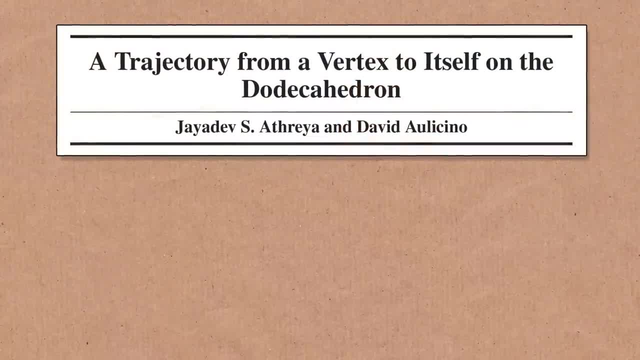 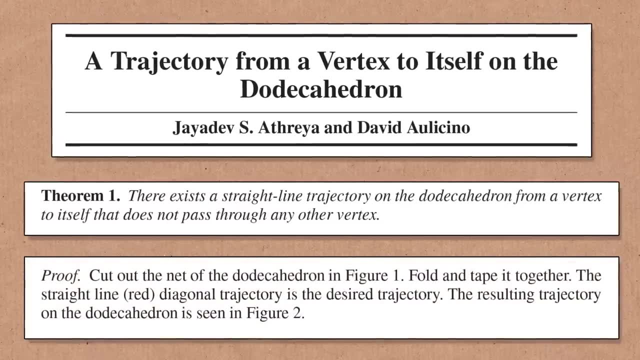 We have a paper, in fact, where it has my favorite proof I've ever written. The theorem is yes, such a trajectory exists. The proof is: here's a picture. Cut it out and glue it together. So apologies to libraries. 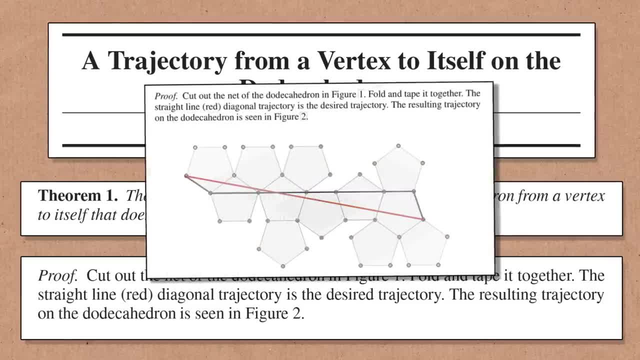 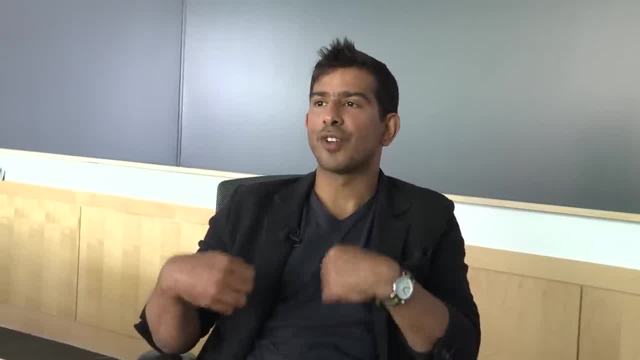 If people are reading this paper, maybe they are cutting this paper out and putting it together. Hopefully there aren't too many mangled copies of the American Math Monthly. But then we also have a really sophisticated and in some sense very satisfyingly complete answer of: hey, not only did we find one, we understand all of them. 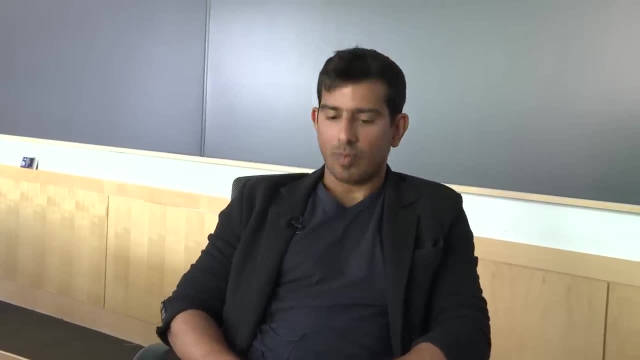 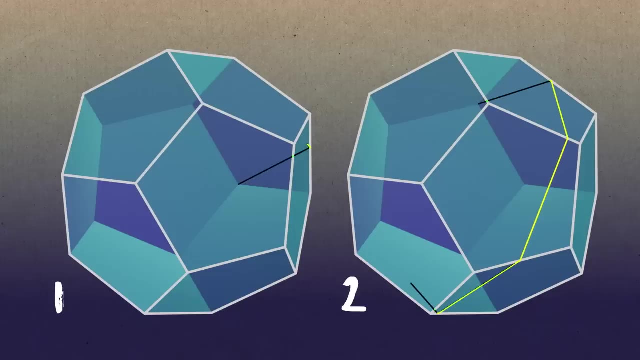 What's the fundamental difference between the 31 different ways? Like if I was using path one or path two, how would I know the difference between the two? So one thing you can notice is path one, for instance, never crosses itself And path two already starts to cross itself. 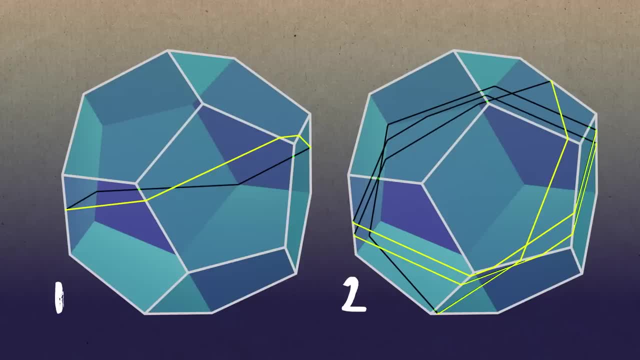 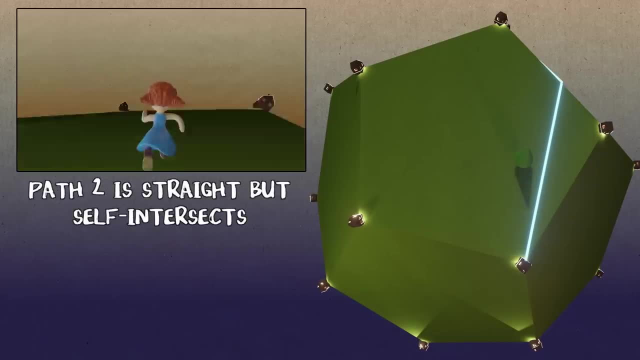 Path one is what's called simple and path two is not. You're crossing over a point you've already crossed over, So maybe you're doing a jogging path where you pass by that same tree twice. That's something that can happen And that's a simple way. 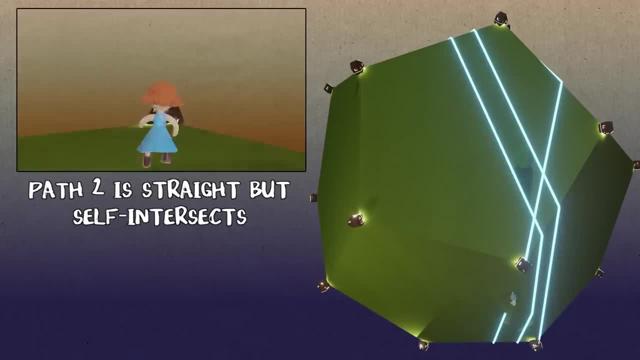 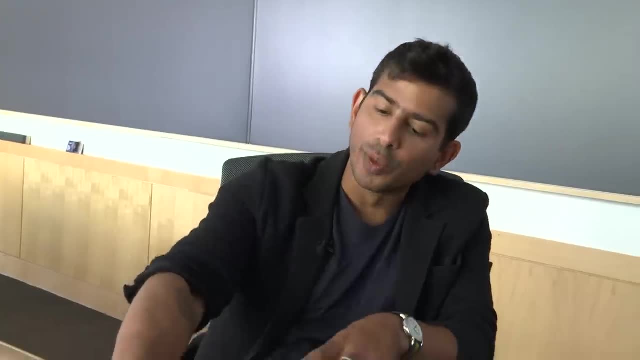 The number of self-intersections of the path is a simple way to maybe tell the types apart. The actual equivalence is what's called affine equivalence. These things are. we're gluing things together with translations, And so you can always just change the whole picture by what's called a change of coordinates. 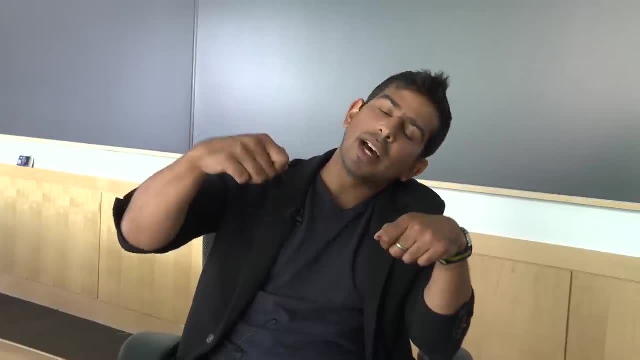 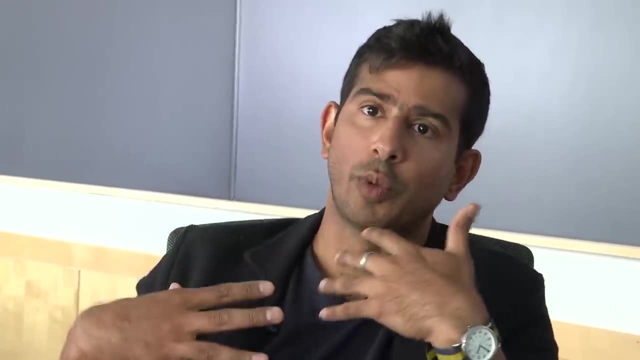 You can stretch and contract and rotate, And if you can do that in a way that takes one path to the other, we consider two equivalent And the number of self-intersections is kind of what we call an invariant in mathematics. That's one way you can tell these 31 apart. 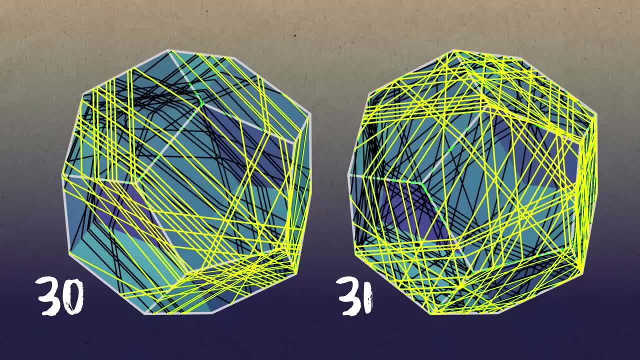 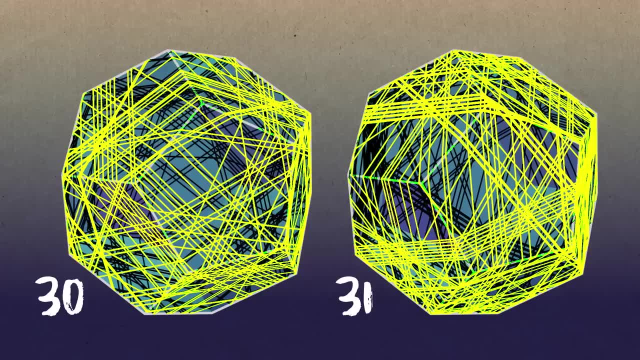 What's it like to have discovered something new about a platonic solid? That's like finding out something new about pi or something. It's one of the most satisfying and exciting things When David Pat and I talked about this, or when David and I first talked about the dead echahedron. 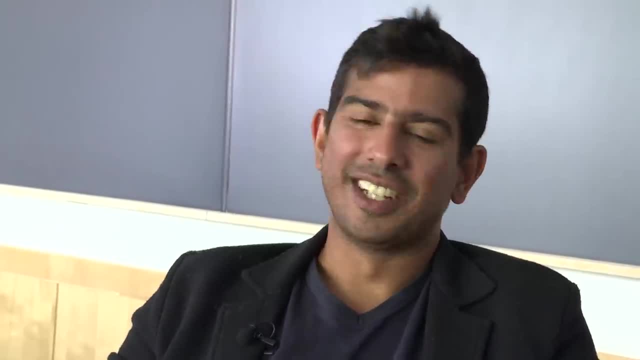 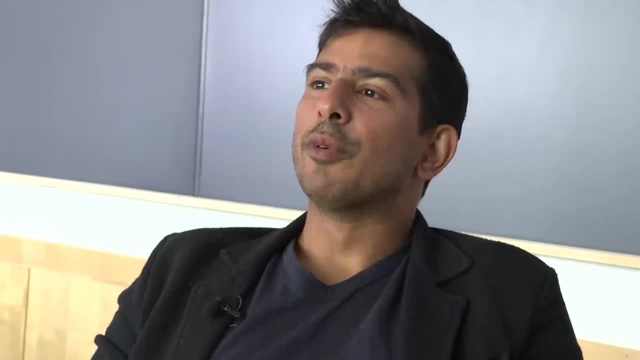 we joked: oh, it would be cool to say something new about platonic solids. What is it? It's an Ecclesiastes. There's nothing new under the sun, But it turns out there is something new about platonic solids. It was really fun because it used mathematics I already knew and I already loved. 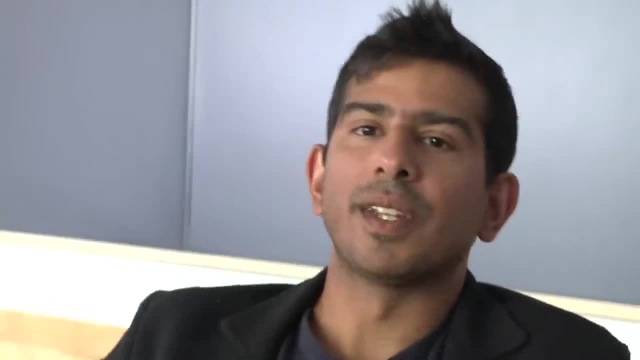 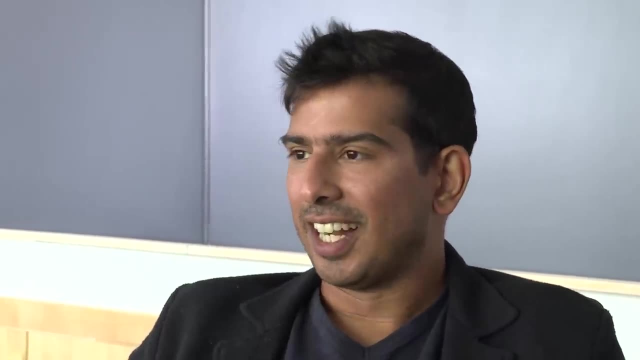 Clearly, I already loved it And I was able to say something new, And I was able to say something that I can share with lots of people. This is something I really care about, And, in fact, we've made activities for schools and so on based on this. 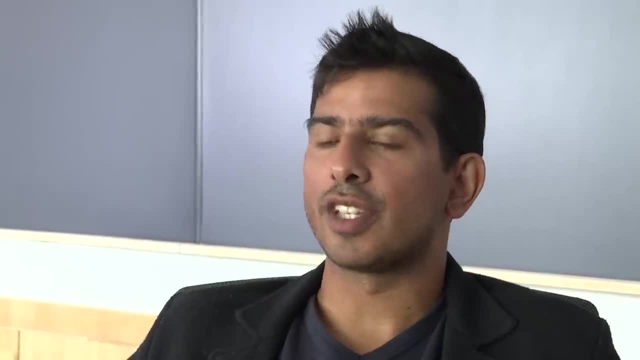 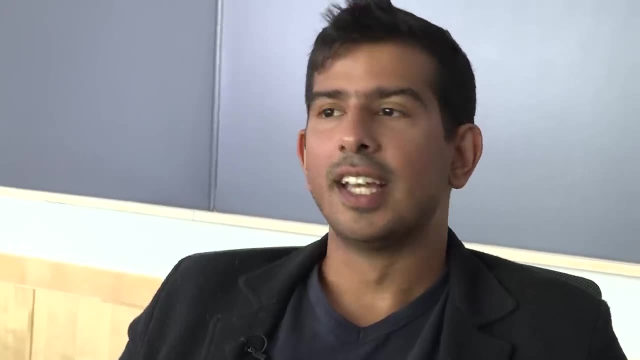 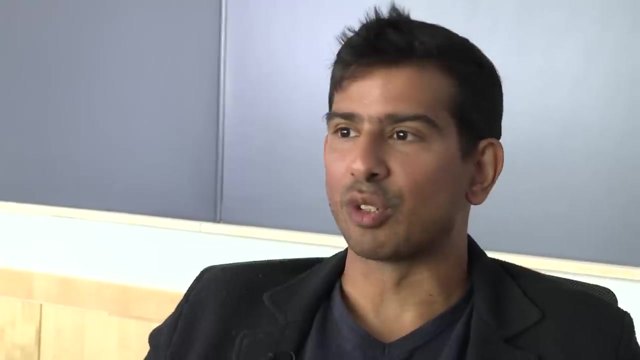 It's something that uses very interesting and very sophisticated mathematics to answer a question that you can state very easily, And so if there's any sort of big point to this is there's still lots of really interesting simple questions out there. Math is something that's alive, that's growing, that's changing. 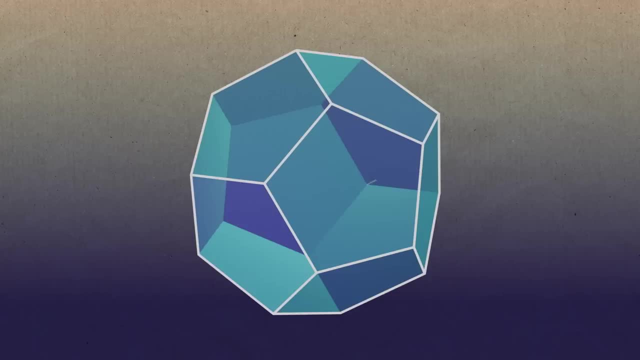 Even the oldest stuff we think about. there's a ton new about it. Have you given any of these paths names, Especially the simple one? Yeah, We should give it a name, The simple one we should. I don't know what we should call it. 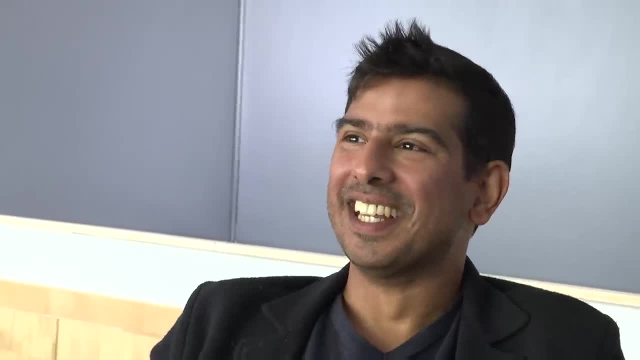 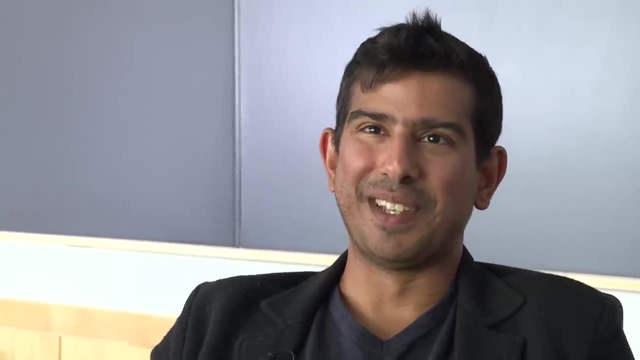 I'd welcome suggestions in the comments, But this one is: maybe we could give them names. Maybe one could be the 5k, one could be the 10k, one could be the marathon, depending on how long they are. I was thinking more, like you know. 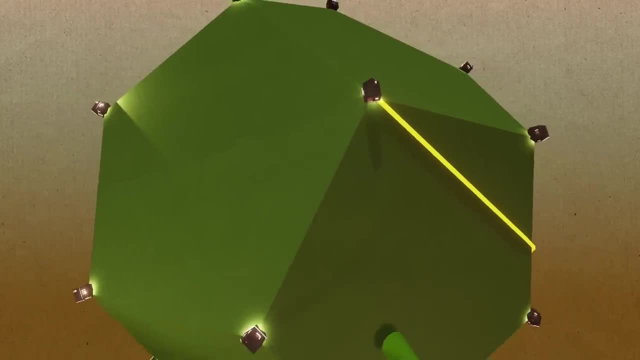 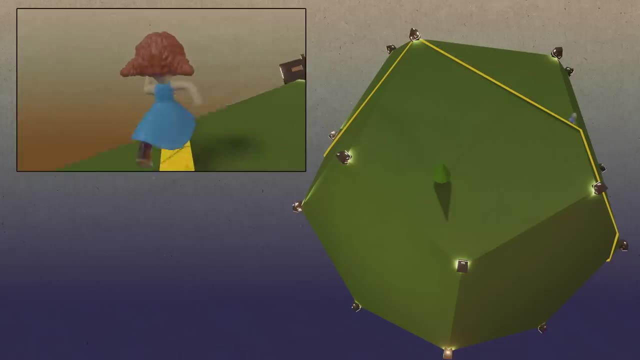 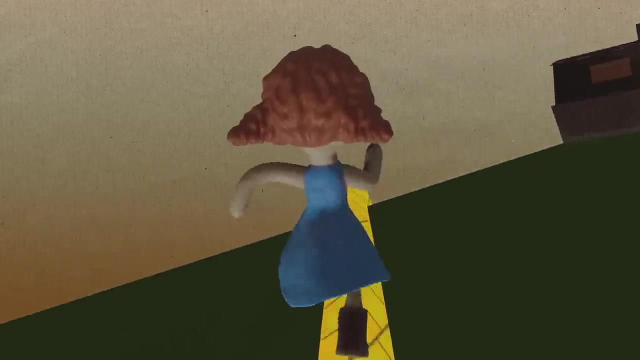 The magic line, or the the yellow, the yellow brick road, the yellow brick road. That's a fantastic, fantastic Eddie. I love that idea. One of the things that's still very wide open is understanding kind of the properties of these lines. for instance, Even that simplest one, we haven't yet computed whether it cuts the dodecahedron in half. 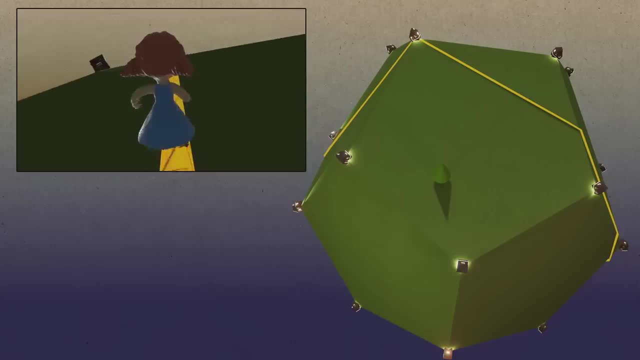 We're to cut the dodecahedron. We don't know the areas of the two halves yet. It shouldn't be too hard to compute. We just haven't done it yet. So if somebody out there that the coordinates are out there in the paper, 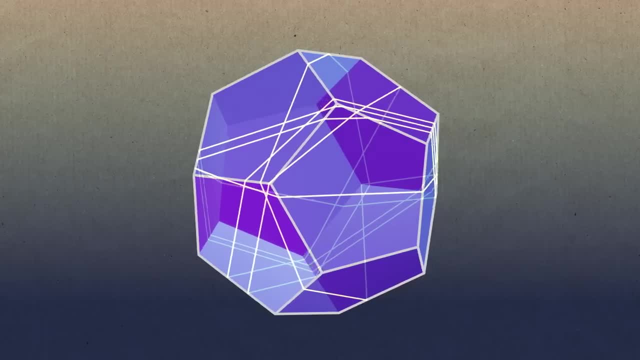 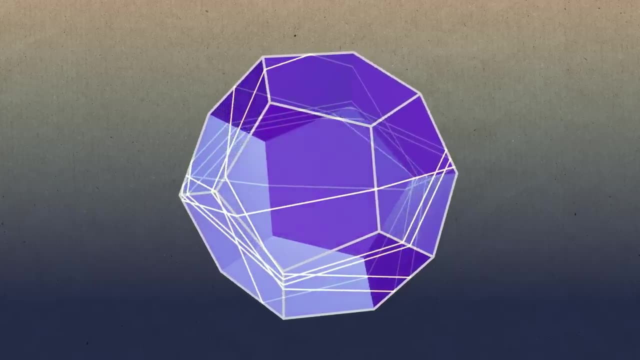 You're more than welcome to compute that and let us know what it is for the other ones. They're going to cut it into more pieces, But what's the kind of the areas of the pieces that's cutting the shape into? what are those shapes look like? 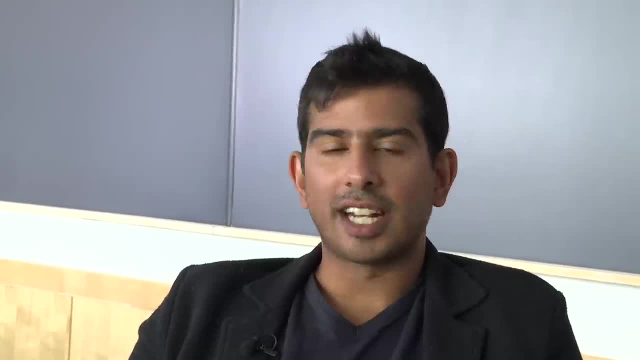 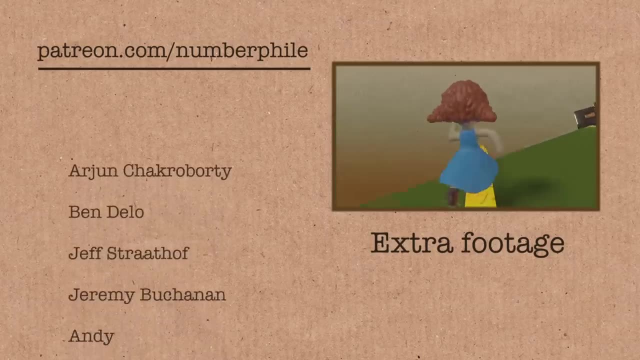 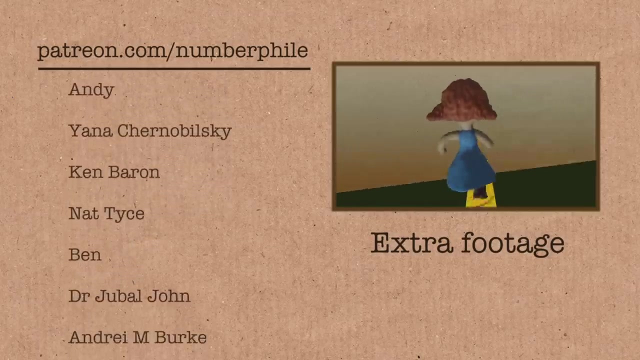 So this is a great thing about answering any mathematical question, is? it actually just generates infinitely more questions. Thanks for watching this video, and a special thanks to our patreon supporters, Including those whose names you see on the screen at the moment. This video was filmed at the Mathematical Sciences Research Institute during one of the programs there. 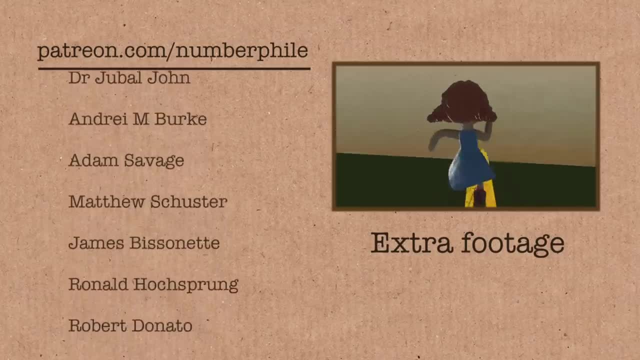 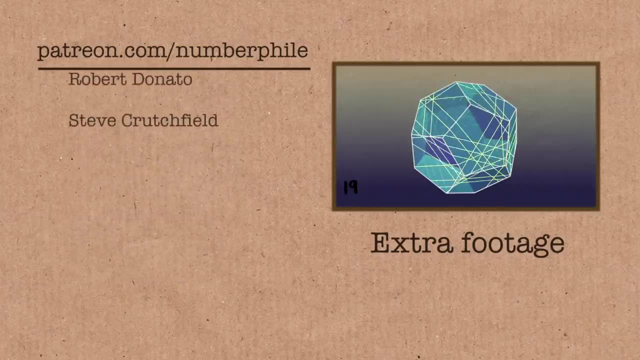 Find out more about MSRI in the video description and to see all the dodecahedrons with their magical paths, Including, of course, the yellow brick road. We've put some extra footage over on Numberphile2.